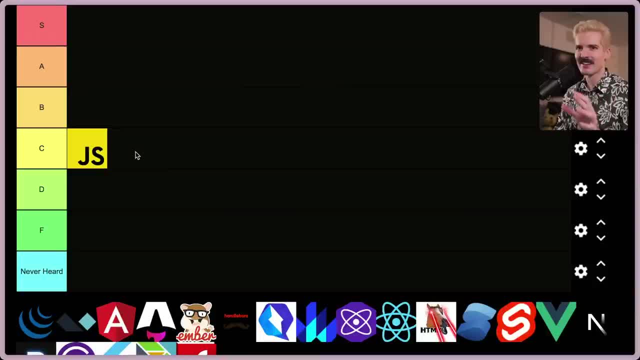 So we'll start with JavaScript as a solid C tier, because, while it's not going to make things worse for you, it's certainly not going to make them better. And now we can rank every other framework against how it compares to just using JavaScript, which is why, obviously, we have to put jQuery in. 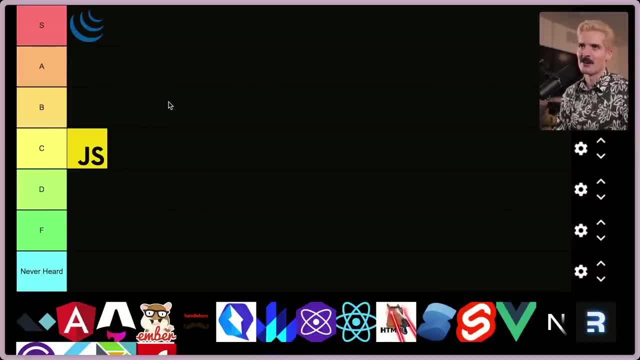 S tier. jQuery is why the internet we have now exists. So yeah, S tier all the way. still a fantastic experience. The majority of websites that people go to still have jQuery on them somewhere. Fantastic jQuery gets S. So what do we go to next? Should we just go in order? Let's. 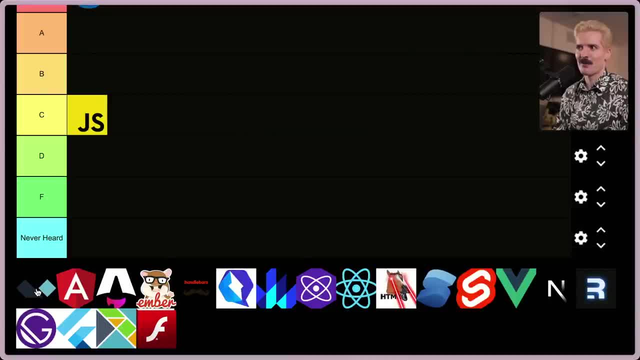 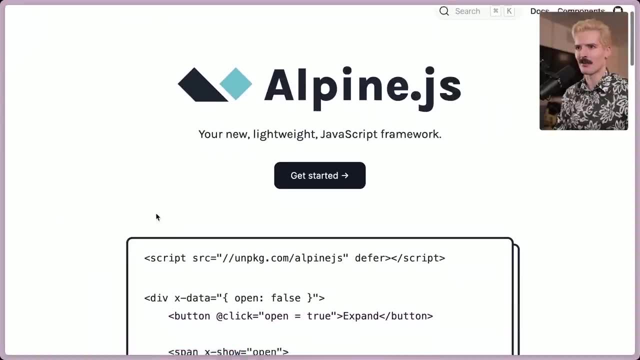 just go in order. This I actually want to know is Alpine, But I have went out of my way to avoid Alpine for a long time, So let's take a quick look at Alpine j s Alpine, your new lightweight JavaScript framework. We love when. 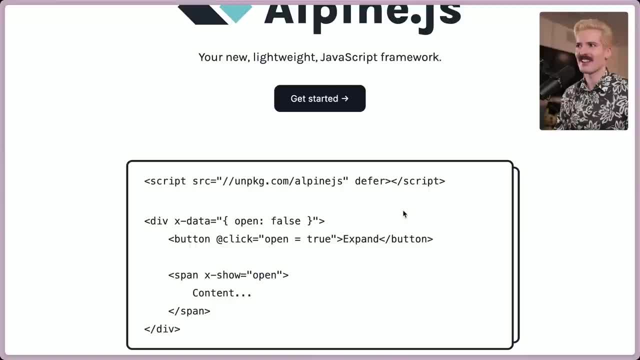 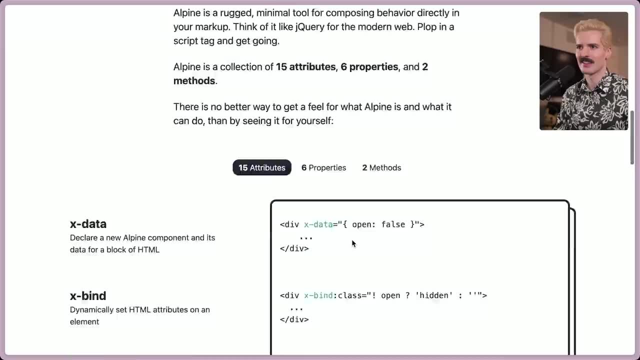 their recommendation for how to set it up is a script tag, That's. that's how you know we're in: deep, simple, lightweight, powerful as hell. I'll find a collection of 15 attributes, six properties and two methods. Declare a new Alpine component data dynamically steady shimella. 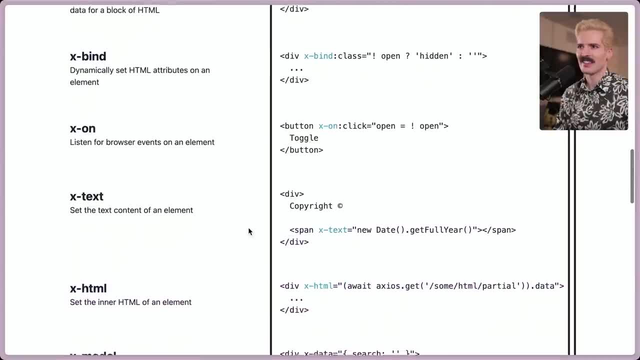 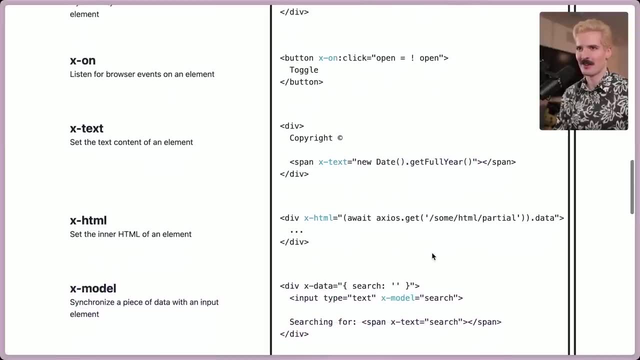 tributes. Listen for browser events. Gotta love that. like putting JavaScript in a string. So I'm just said it's like Mini view, It's like a cursed version of you. Oh, xHTML. That sounds familiar to something we'll be talking about in a bit It. 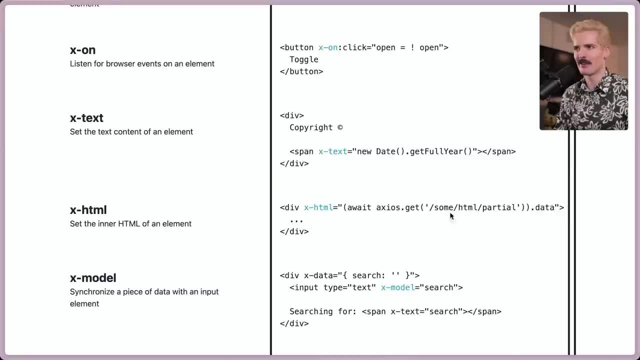 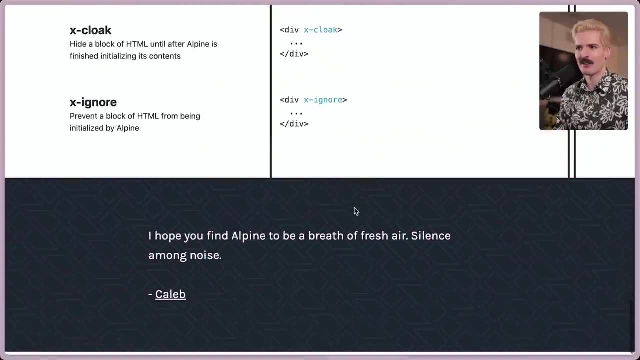 looks like what this is doing is. it's setting the HTML contents to whatever this ends up returning. just pretty cool. Can see how this would be useful, having a transition elements and all of this, But it all is part of the HTML. hope you find Alpine to be a breath of fresh air, Silence among. noise, Being that it's basically view syntax for a mid version of HTMX. I'm pretty much, I'm pretty happy with this. I'm pretty happy with the HTML, the HTML that we have, the HTML version of, but all of the HTML, html. The way it works is that it's it's getting it's getting really rich with and 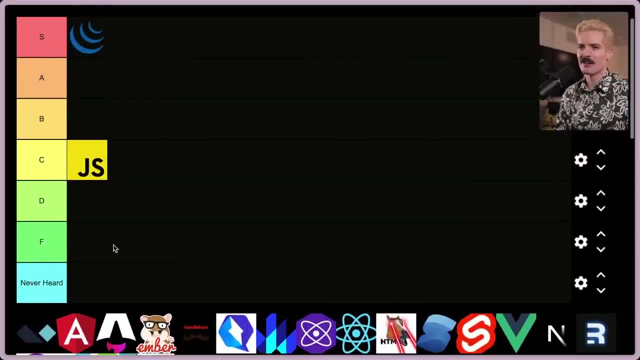 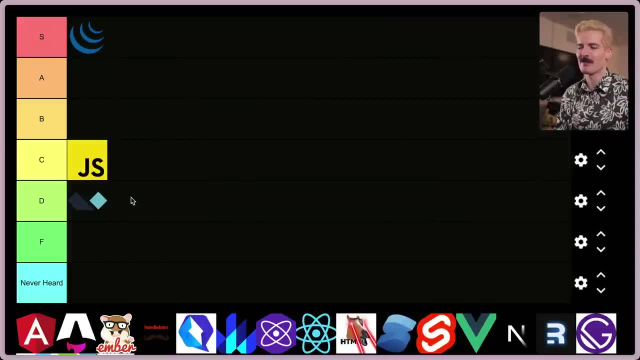 Being that it's basically Vue syntax for a mid version of HTMX, I'm putting that in a solid between C and D tier. I feel like it would have been higher before HTMX became relevant, So I'm putting a D for now. Now we got to talk about Angular. Angular's had a long journey. 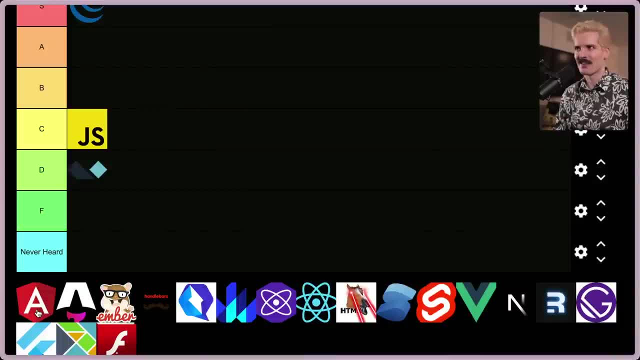 And from AngularJS to Angular alone. that transition was nuts, But it also helped kickstart this new component-based web and allowed for much larger web code bases to become the norm- Most of the first giant websites with hundreds of developers contributing lots of dynamic. 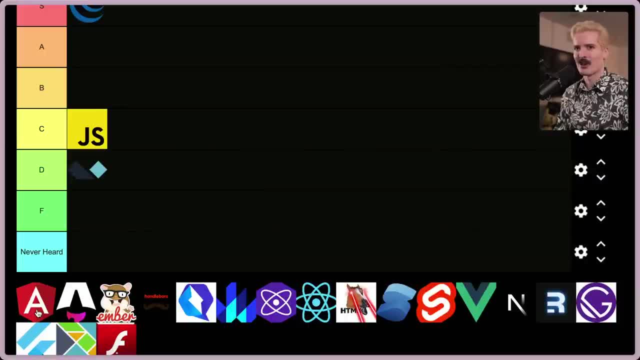 features every day were in Angular. That said, I have never enjoyed myself writing it. It is one of the most painful frameworks to work in that I've ever used. I hate almost every implementation and design decision made within it. I want to give it an A in spirit and a D in use. 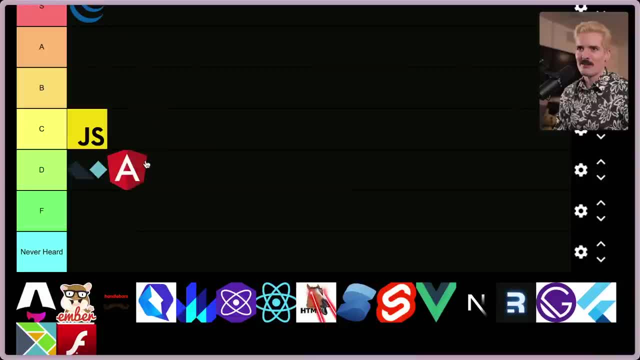 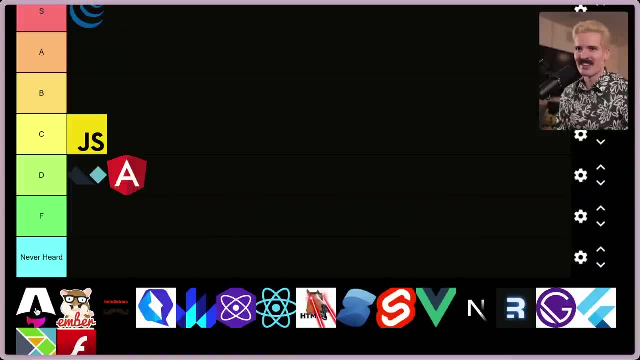 For impact and importance. it's an A, But please don't make me use Angular. Okay, Astro being in use Here is a scam, Because many of you guys know this. Astro is not a framework. Astro ships no code that runs in your browser. You can use it to generate HTML on a server And then you can. 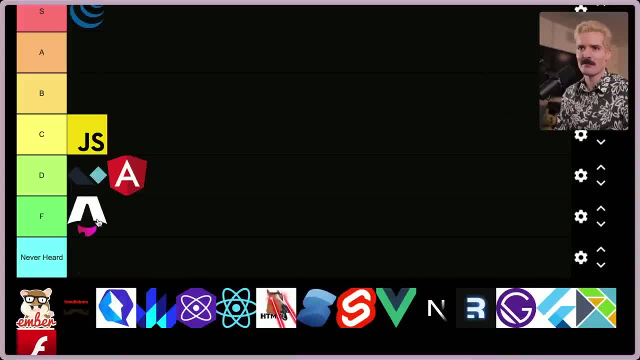 mount like a React component or whatever in it, But for being an imposter F tier. the whole, like web transition stuff, makes it a lot more possible to pretend that it's a JavaScript framework. But it's not. There's no router, There's no JS running in the client. It's not a real framework. Get out. 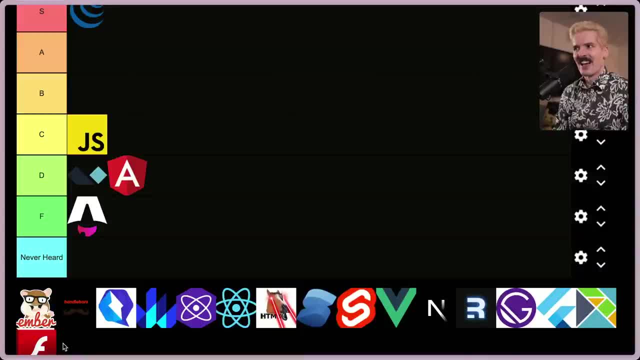 of here. Oh no, Ember, I forgot this was in here. I do my best to forget about Ember. Brief story time. Ember is a big part of why I didn't think I liked web development, Because when I started at Twitch, we were still using Ember for the front end and 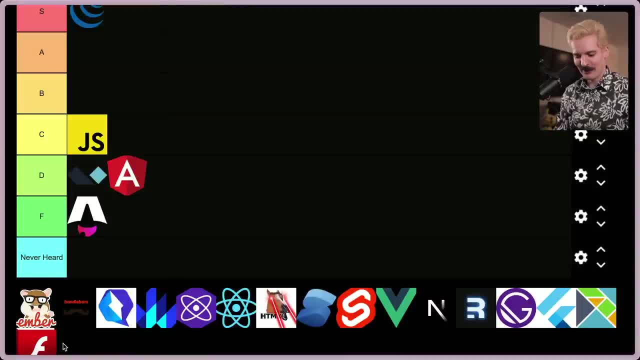 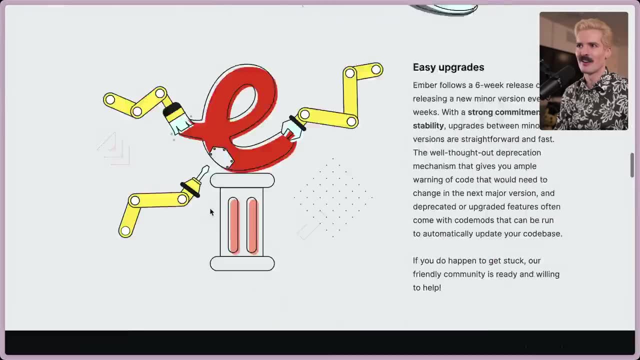 Rails for the back end, And I hated every moment of it. I want to show you guys some Ember syntax, just so you can understand that I'm not insane here. If you've never actually looked at Ember code before, there's a reason they don't put any on their homepage: They don't want to look at it. 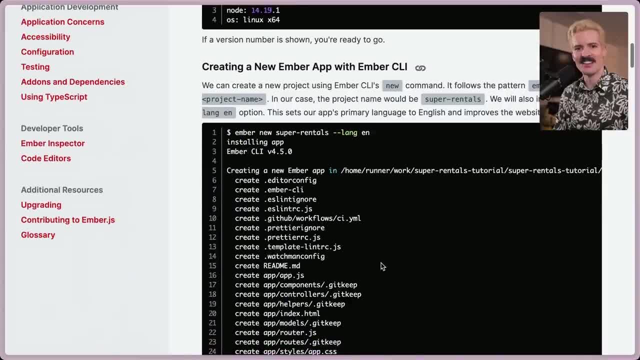 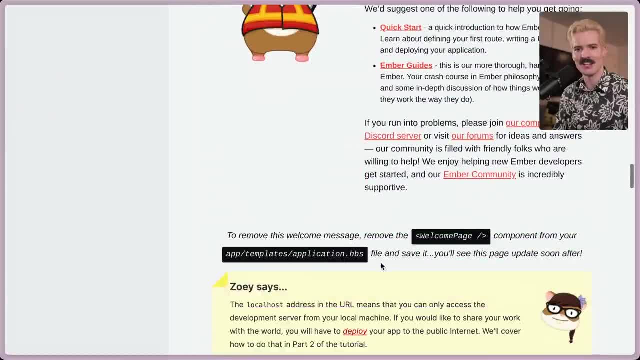 either. Okay, so the first thing you should know about Ember is that they're really good at code gen. So, like, when you want to make a new route or something, you run a script or a CLI command and it generates that new pile of things you need. They also have their own crazy templating. 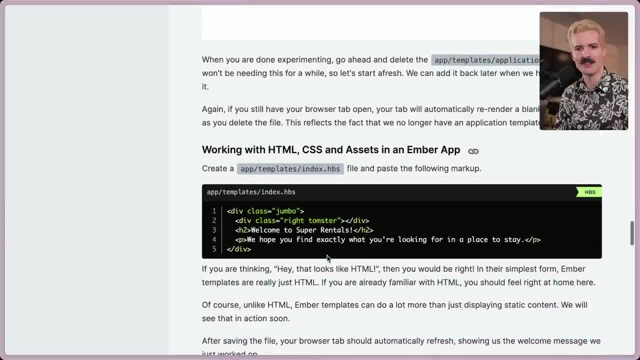 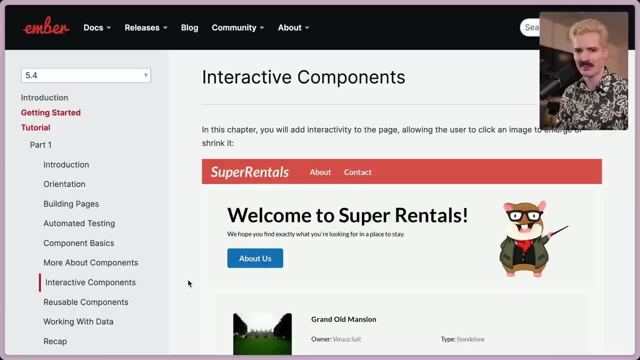 syntax HBS. It's handlebars based, but they've done some crazy stuff to it. Interactive components: Okay, we have been through 1,, 2,, 3,, 4,, 5,, 6, 7 pages And now, after writing, two dozen unit. 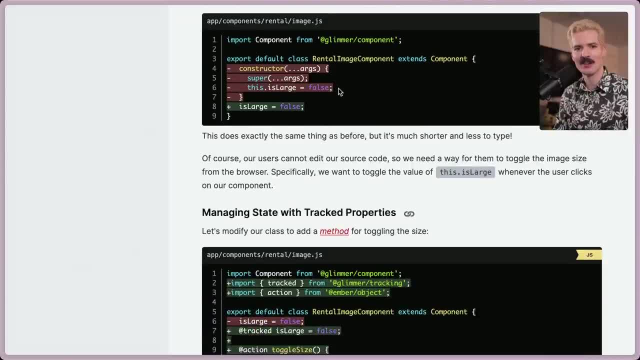 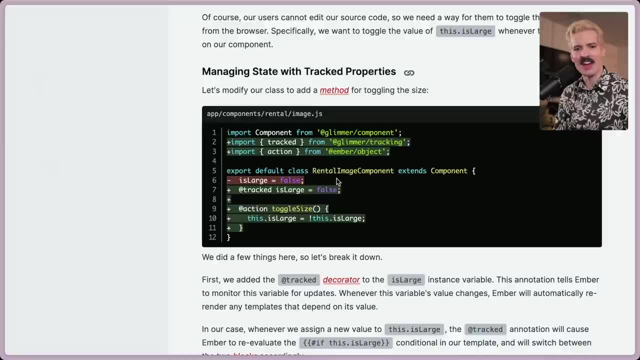 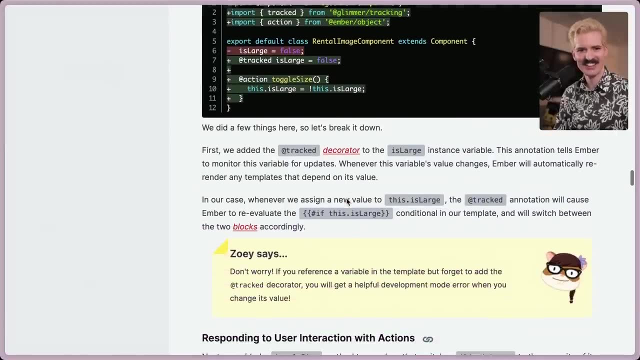 tests. we might finally have some JavaScript code, which obviously is classes, Because why wouldn't it be Managing state with tracked properties. You have to delete that and at tracked decorator, which now means you have to use one of their crazy compilers that handles these decorators. If you reference a variable in the template but forget to add it, 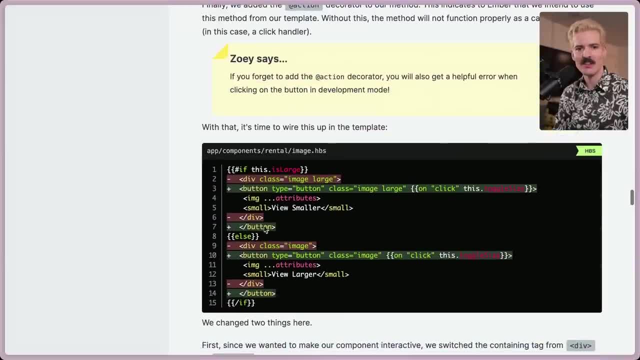 to at tracked, you'll get a helpful development mode error. So now that you've bound that as tracked, you can now access this, And once you want to actually do the toggle on, click this dot toggle size. you have to combine handlebars. 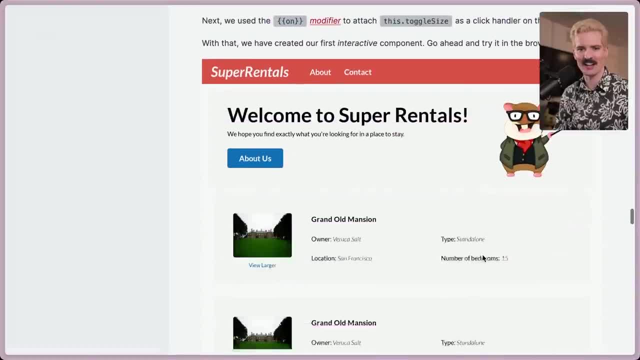 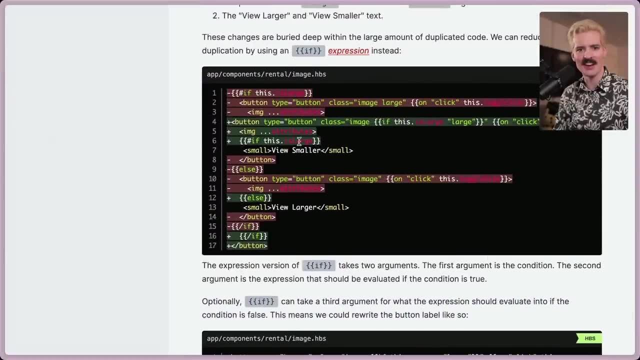 It's kind of like a syntax with their weird binding bullshit. It's horrifying And there's like no deterministic anything between them. You basically need dev mode to tell you if you forgot stuff. If this dot is large, show, else God forbid, your JavaScript code and your template aren't in. 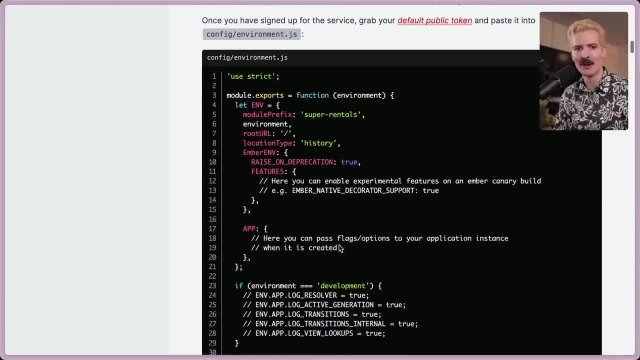 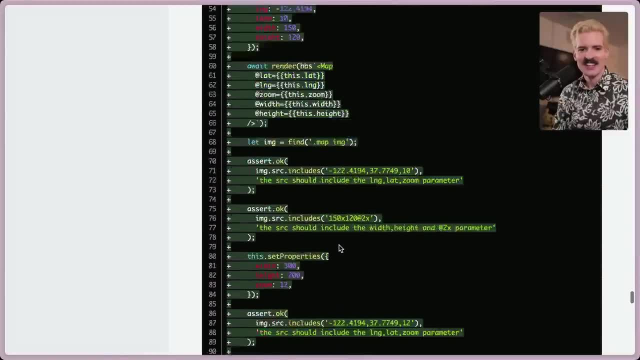 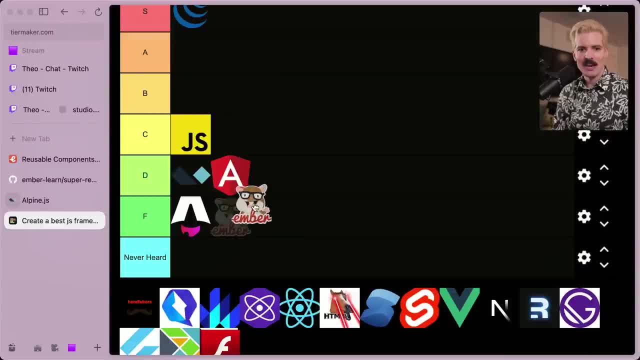 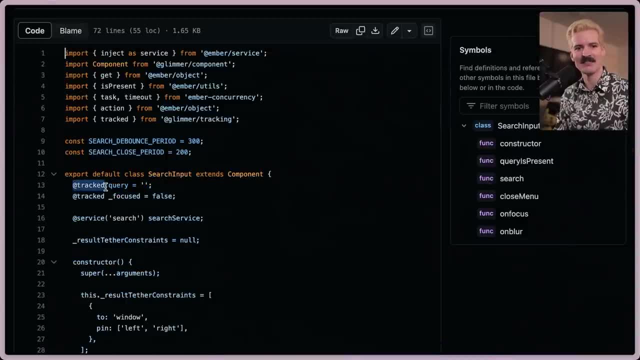 I don't care anymore. Ember is going where it has. hurt me F tier. Somebody just said GitHub doesn't even know how to highlight Ember code. I want to see this. That's hilarious Because, again, putting decorators in front of a variable isn't really a JavaScript thing. So most JavaScripts, and even 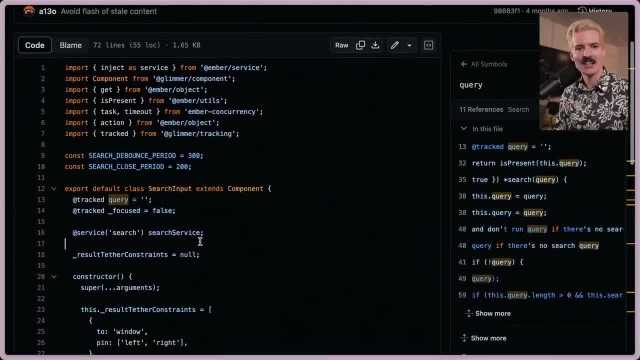 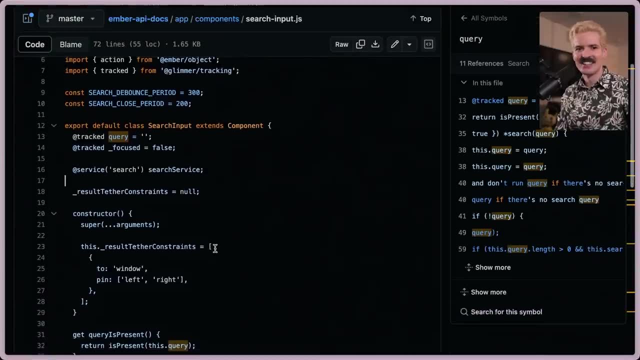 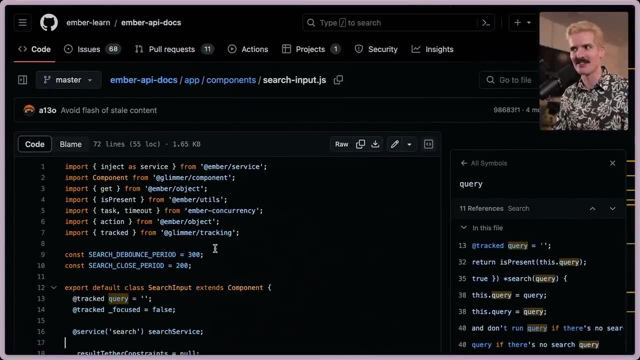 TypeScript parsers are going to entirely screw up the highlighting, Like: the argument against JSX is that it ruins your JavaScript and it's no longer JS. What the fuck is this then? Like, come on, You can't say the reason you didn't do JSX is because it's not JavaScript, and then do this. 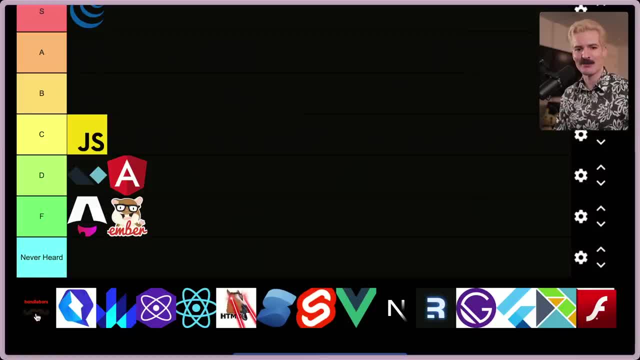 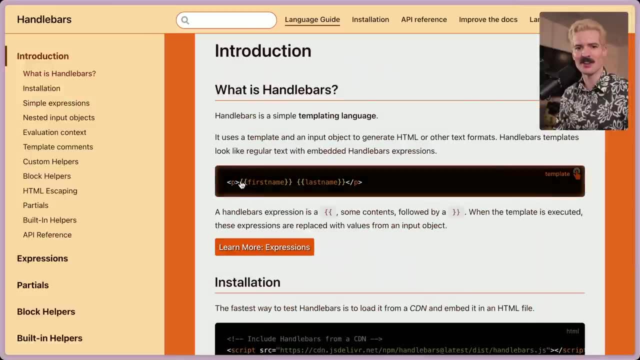 shit instead. That's enough crapping on. Ember. Got to talk about some real frameworks here with handlebars. For those who don't know, handlebars is a templating language. It's called handlebars because you use brackets all the time to embed values, like all of the time, And it's like the. 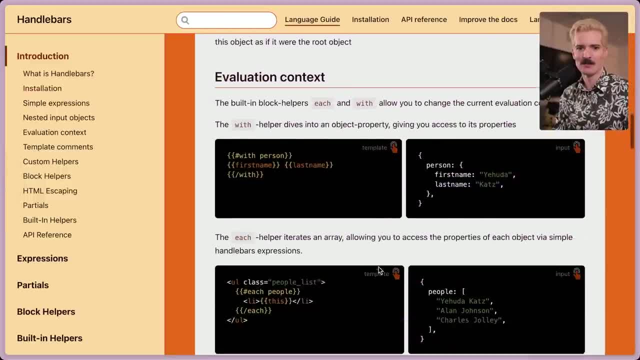 handlebars are the little curve like a mustache, which is also their logo, Clever branding. But the point of handlebars is: you want to be able to do it, You want to be able to do it, You want to be able to. 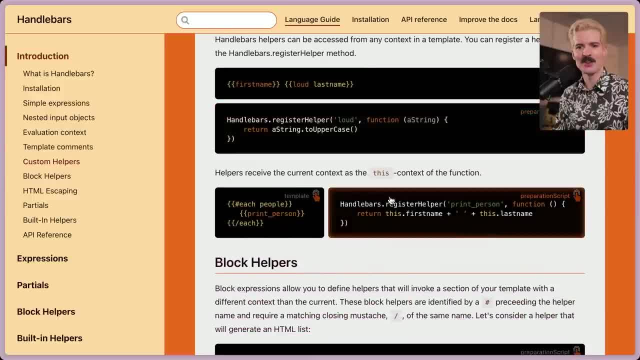 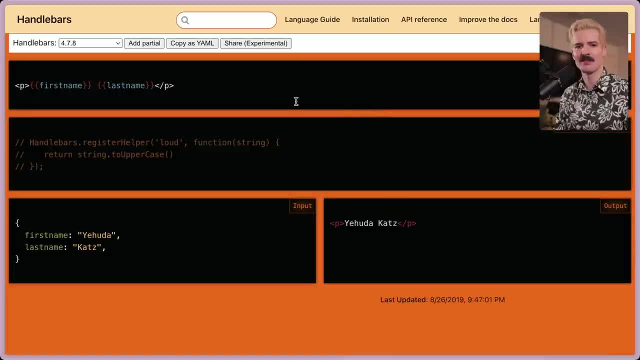 do it. You write code that requires specific things, And then you can feed it values from JavaScript and it will handle all of the registration there. This is a handlebars template. This would be an HBS file, or you can technically write it in your JS files too, And 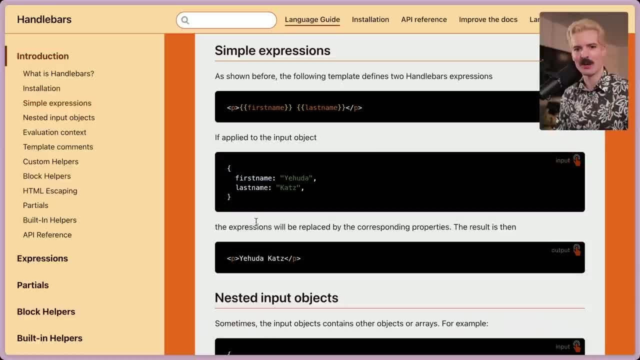 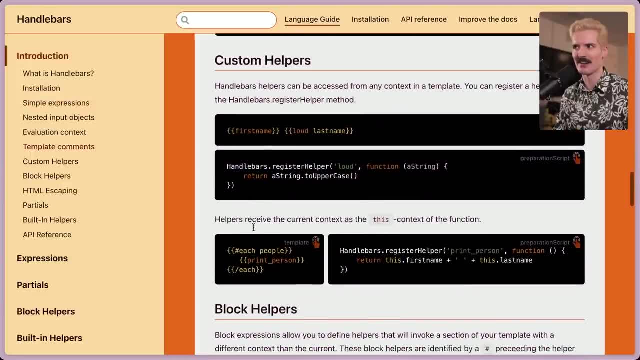 then you run the handlebars framework, pass it the object with whatever you want and then it will render. So it's like an interim step for templating your HTML to pass it values. It's important for its time. The idea of a standard HTML template is that it's going to be able to. 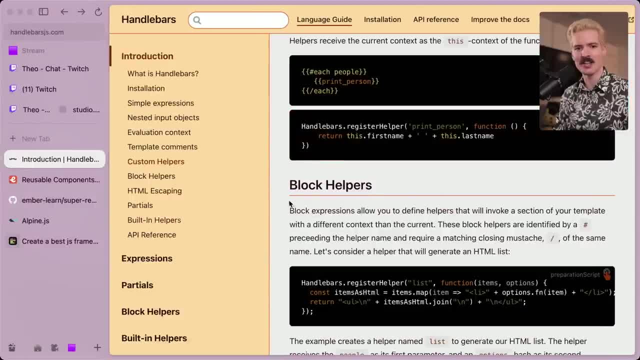 render it. It's going to be able to render it, And so the idea of a standardized way to update and render HTML from JavaScript was a really important concept. It was almost like the opposite side of what jQuery was doing. which jQuery thing was given. You have this HTML already. We're going. 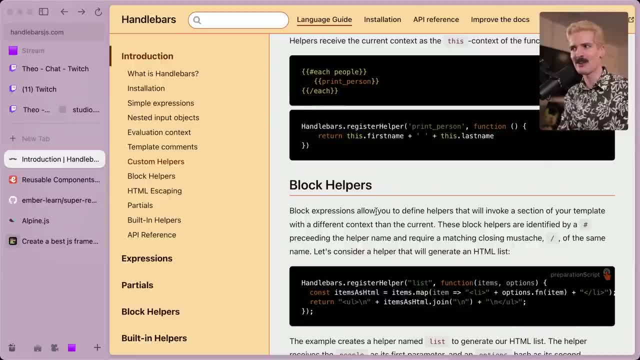 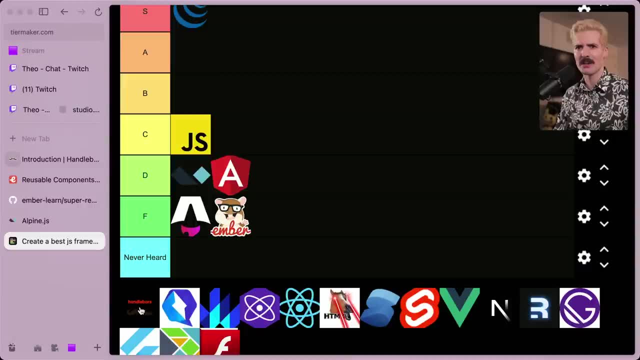 to allow you to bind behaviors to it. Handlebars is. here is how we generate the HTML. Really interesting concept. It definitely helped us, as a field, rethink the relationship between JavaScript and HTML. So I want to put it slightly higher than Vanilla JS for that. 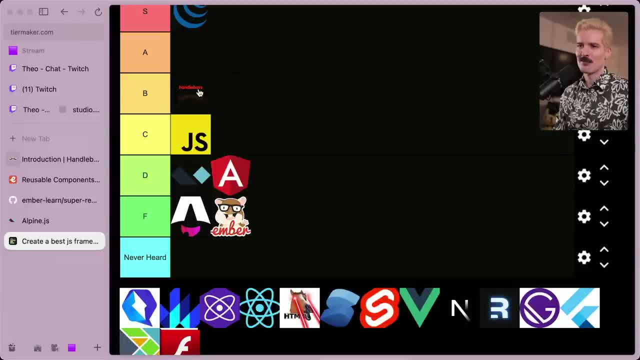 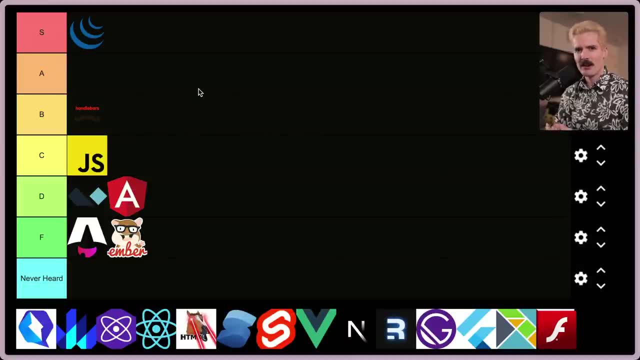 reason. Let's do it Slightly better than Vanilla JS. Oh boy, now we have to talk about Quick. If you're not already familiar, Quick was created by Mishko, who was the original creator of Angular. There's a lot of problems that modern JavaScript frameworks have introduced to the web that he is. 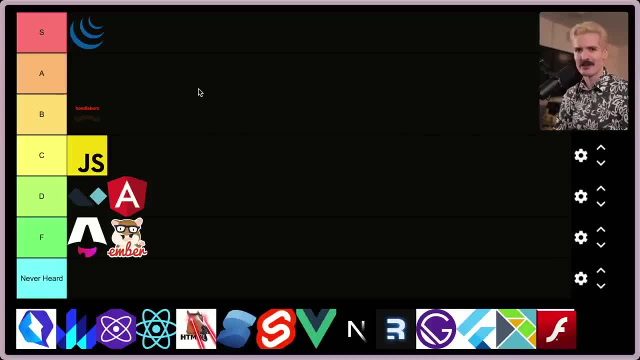 really upset about and probably feels some amount of responsibility for, as the creator of Angular. Those problems include loading way too much JavaScript time to interactive, getting way slower over time, data waterfalls causing multiple elements to pop in synchronously instead of all flowing together at once. A lot of these types of problems have made the web worse to use. 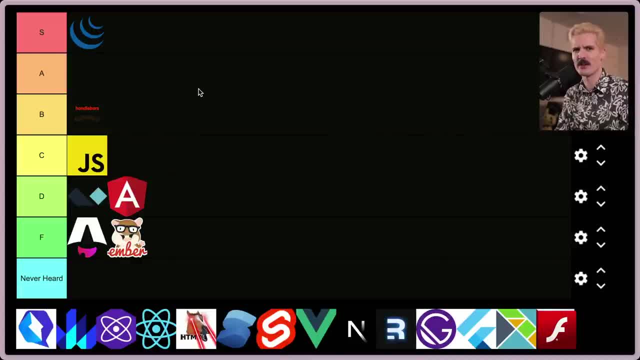 especially if you have a bad internet connection, And he's built Quick to target those problems. The thing he's focused most of Quick's branding on is the concept of resumability. Most other JavaScript frameworks have an idea of hydration, which means given some HTML. 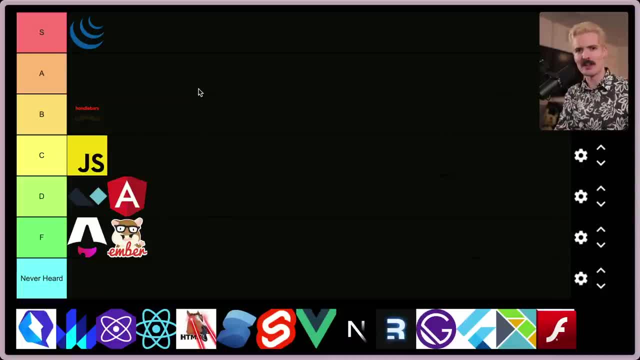 and then, given some JavaScript, the JavaScript will catch up to the current state of the HTML by re-rendering a lot of the parts, And this takes some time If you have a giant HTML file and then it takes a while for a giant JavaScript bundle to load and then it has to. 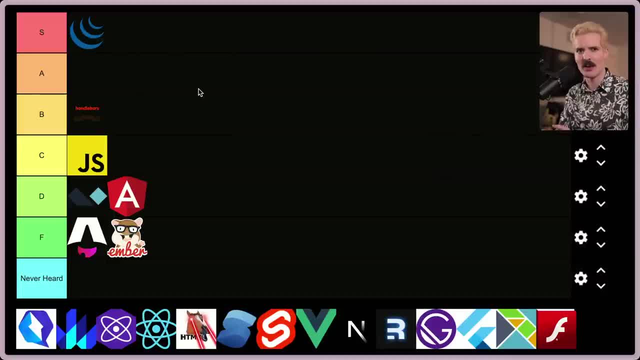 process in your browser, and then it has to run, and then it has to attach to all the elements in your browser And then, finally, you can now interact with buttons, And if you clicked a button in that window, it just wouldn't work. Quick's focus on resumability means that it can. 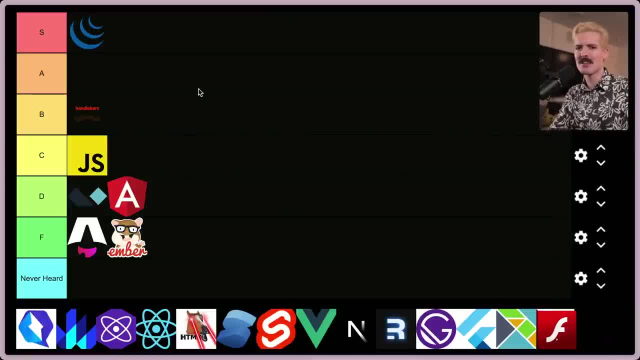 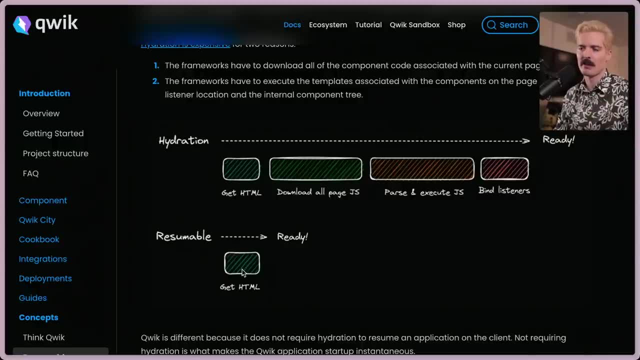 skip a lot of those steps, embed a minimal amount of JavaScript and immediately bind to a button. Here's a diagram from the Quick team, obviously made in Excalibur. quality Excalibur users meant to showcase how resumability gets your HTML ready faster than with traditional hydration. 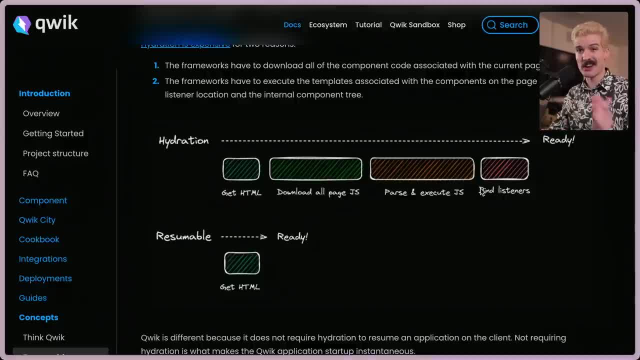 where you have to download the JavaScript, parse and execute, bind the listeners. But there's a lot going on on the other two sides of this And I find that for the vast majority of users, the amount of time all these steps takes is pretty low. And if you only have to download, 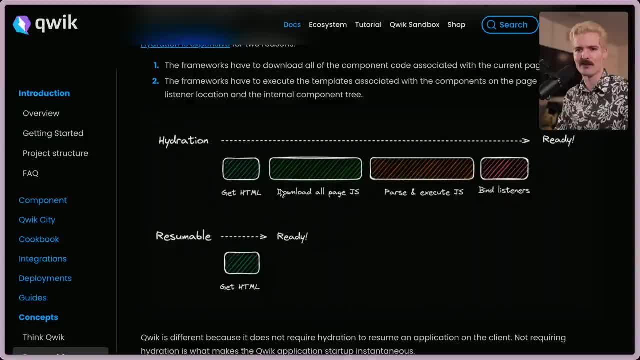 that JavaScript once, then most of this gets eradicated for future visits. Resumability is, in my opinion, not that big a deal, And the only place you would feel it is the amount of time it takes from when the page first loads and shows you content to when you first click a button. 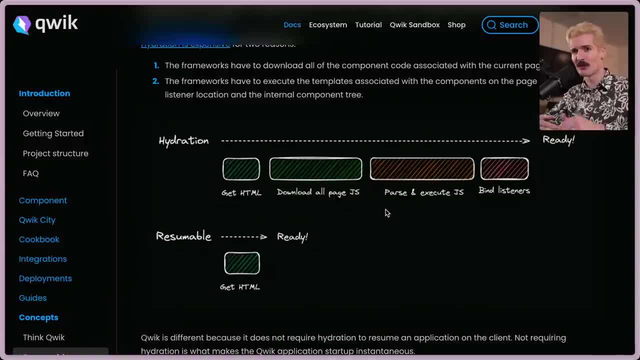 So unless you're opening a page and immediately clicking buttons, and you also have never been to that page before, I don't think it's that big of a deal. So this is where I don't necessarily Quick's focus on its differentiators is as valuable as it has been pushed, especially now. 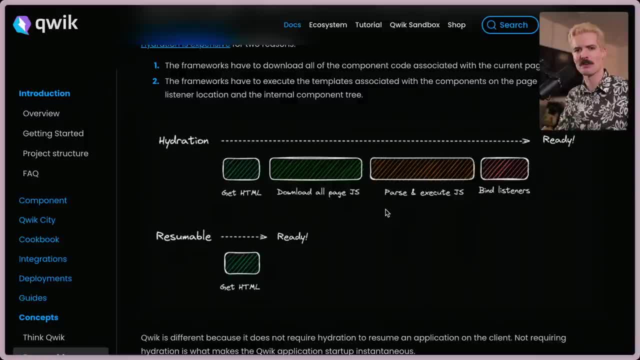 that other frameworks like React are catching up and having hybrid hydration models where some content doesn't need JavaScript at all. Quick has forced us to think about these things more, But the more I've thought about them, the more I realize hydration isn't too big a deal and is 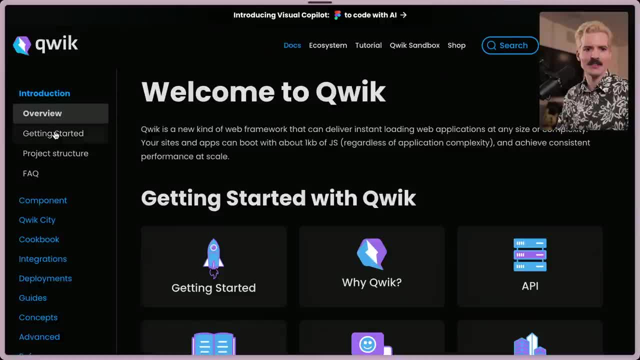 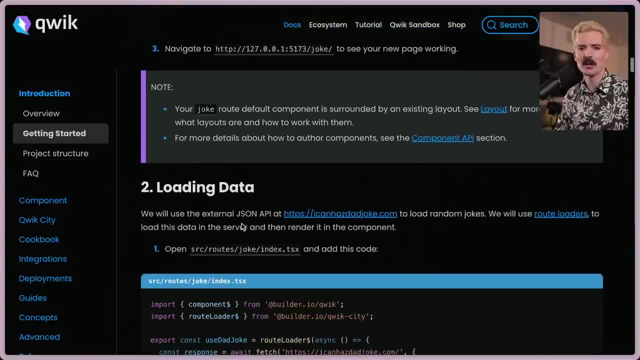 getting better anyways. But if we look at the actual experience, this should look a lot like React to you. Big difference is the component dollar sign code that you have to call in order to basically tell the Quick framework. hey, by the way, this is a component, Everything else. 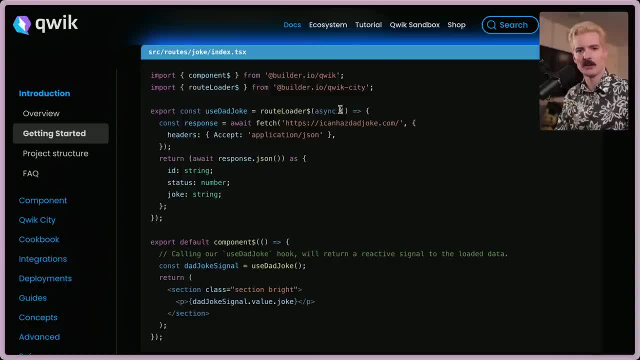 roughly how you would expect here is using Quick City for data loading, So use dad jokes meant to be a similar to a hook in here. you can just call a sync code because we're wrapping it with this route. loader helper has an async function. it fetches some stuff and then it returns the JSON. 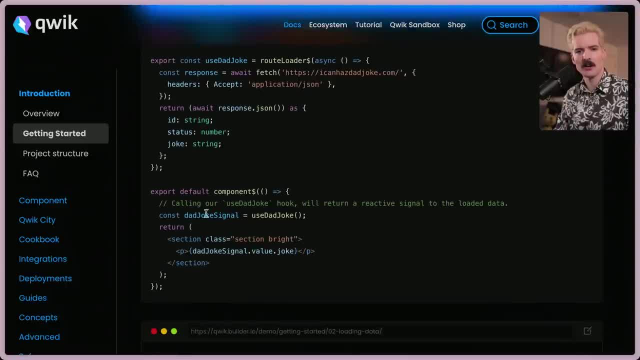 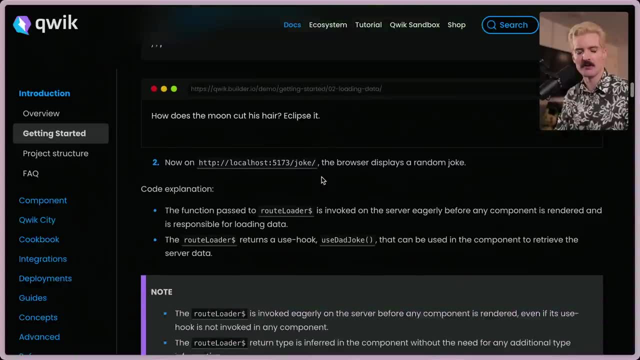 parsed with this type And now in an actual component we can call, use dad, joke and return some stuff. And now this page won't load until that content is done because this will run on the server through the route loader. You can also do an action which is the opposite way. 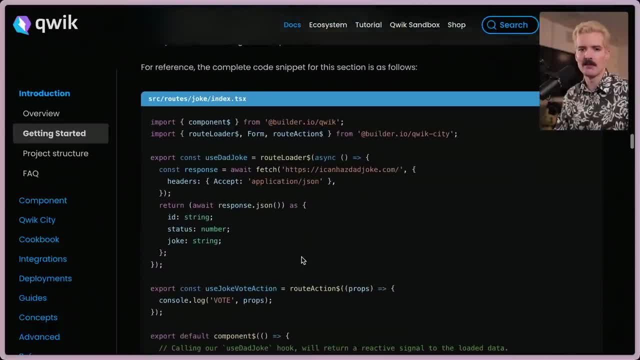 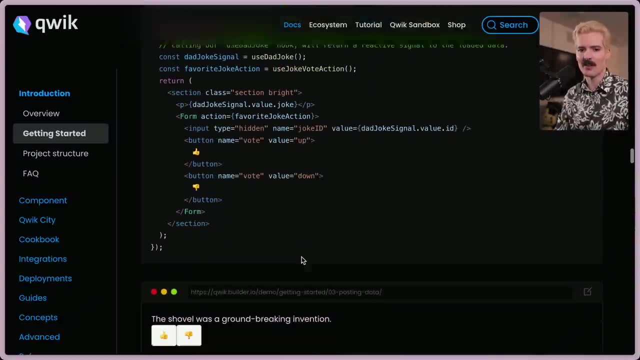 what you'll start to see with Quick is it's this weird hybrid of something like solid and something like remix and react, And the result is seemingly pretty cool, But a lot of the concepts and a lot of the things they push around like JavaScript, not appearing until you scroll to the element that 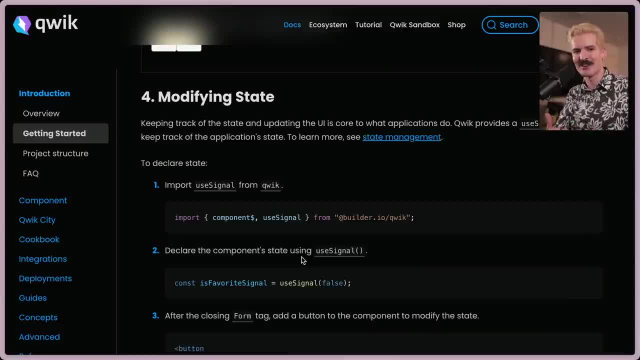 needs it, like not necessarily knowing which JavaScript is or isn't going to be in the browser when you actually load the page. the actual DX corks around this have been a bit weird to get my head around in the bit of time I spent with it And I don't think the benefits it introduces are. 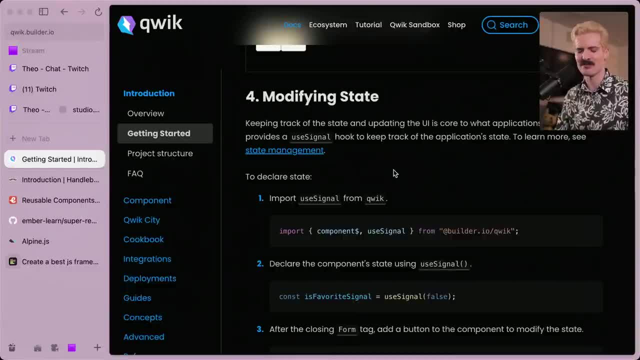 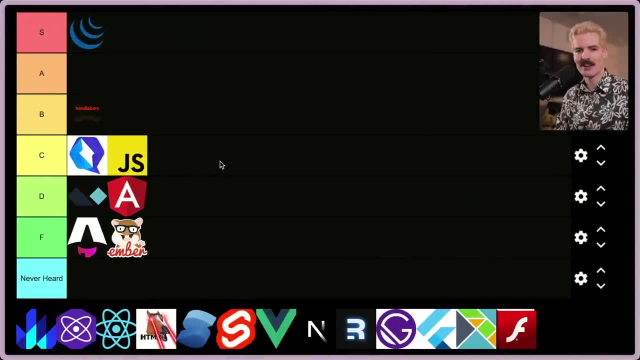 worth it. That all said, it's really cool to see A framework taking these problems seriously and pushing the web standards, And for that alone I have to put it a little ahead of JavaScript. quick, slightly better than JavaScript. Speaking of slightly better than JavaScript, lit, if you're not already familiar. lit is the framework built. 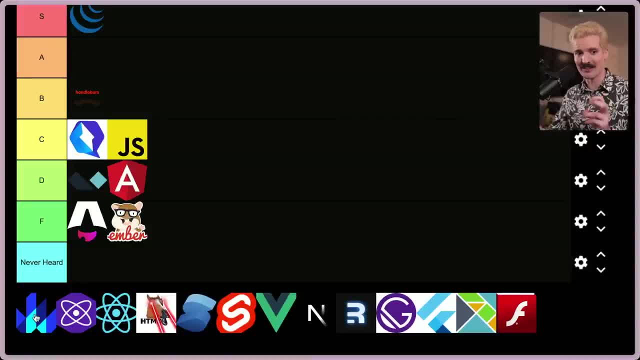 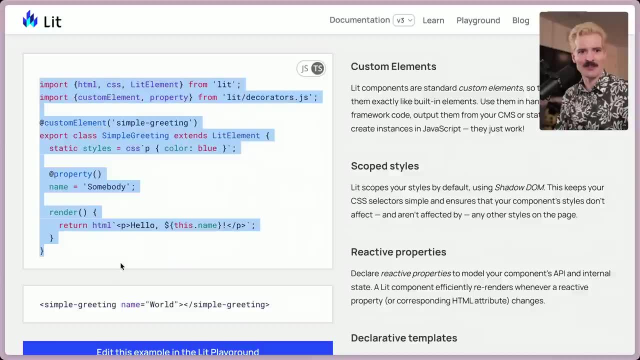 around web components. they wanted to take the actual web standards and try to make them usable, because writing a web component from scratch it sucks. It's really not fun. So this is a vanilla JavaScript version This theoretically would just run in the browser, which is really. 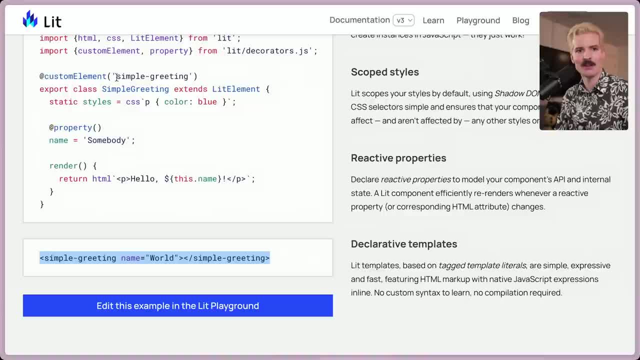 cool. And now, more importantly, you can mount this custom element that you've bound as simple greeting in your browser as a traditional HTML element, and it will just work. That's really cool. I don't think any of the other frameworks here have that capability, where you've now created an element you can access in the. 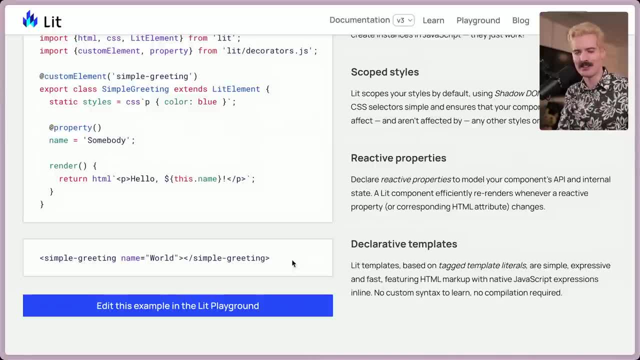 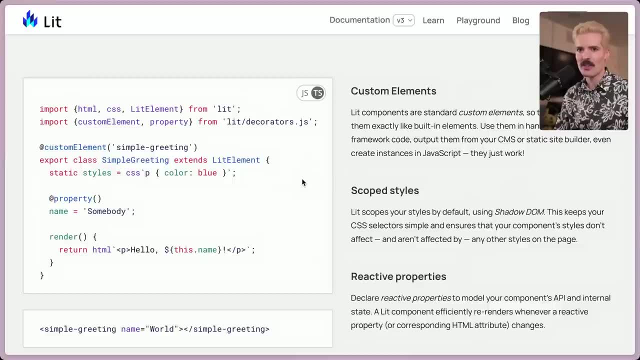 browser. But that's the goal of lit is to be as like traditional HTML and JavaScript and the browser as possible, using all those standards, but giving you this abstraction on top that makes it actually somewhat pleasant to use. Let's a weird thing to use for your big projects And I wouldn't. 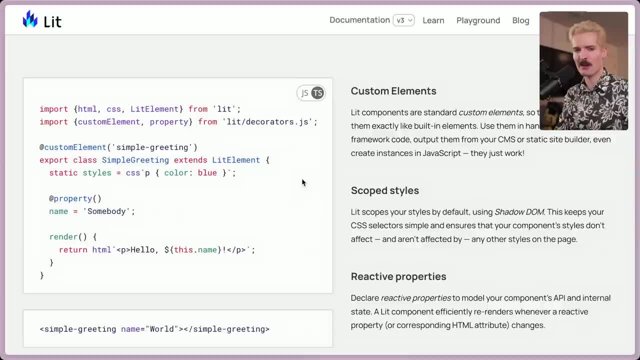 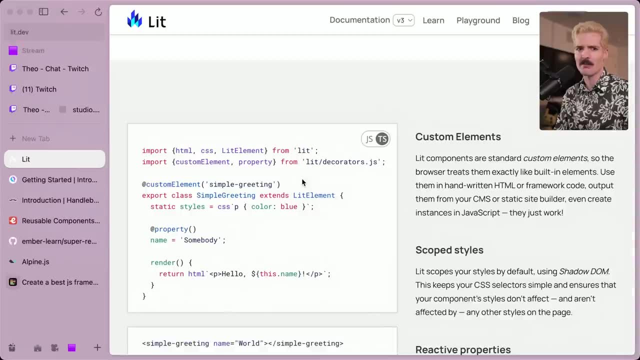 enjoy working on it, with a huge team trying to build this gigantic platform, But if I wanted to have an element that could be reused on future projects, or just take one part of my blog and make it interactive. let's really nice for those types of things And again, I think 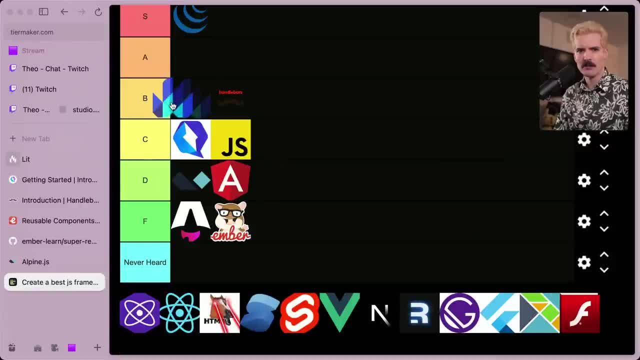 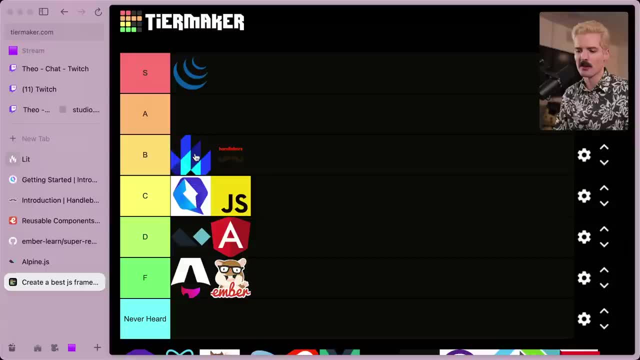 it's quite a bit better than vanilla JavaScript. I would actually say it's pretty similar to handlebars, although I would hate using it less. So I'm between B and A tier for lit because it's solving problems other things don't solve, But I also wouldn't use it for large. 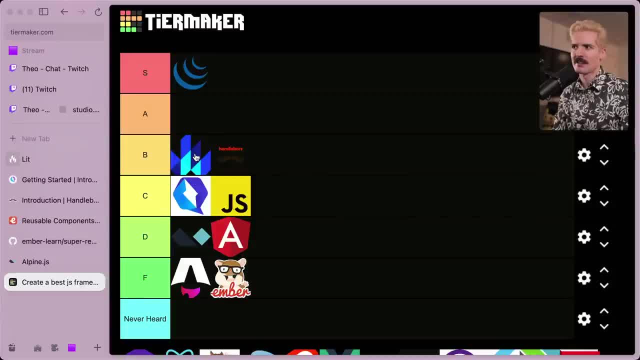 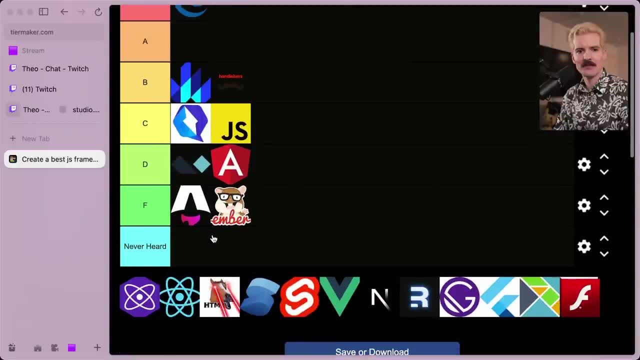 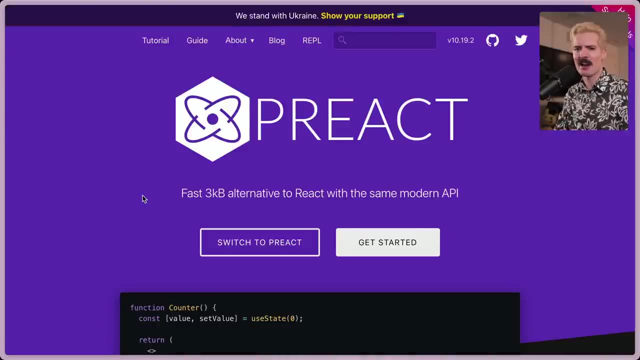 things. I will appeal to chat. we feel an A or B tier for lit B is like B is the consensus. We'll leave it in B. Cool On the topic of web standards and working really hard to comply to them. We have pre act because you haven't heard of react before. It's the fast alternative to react. 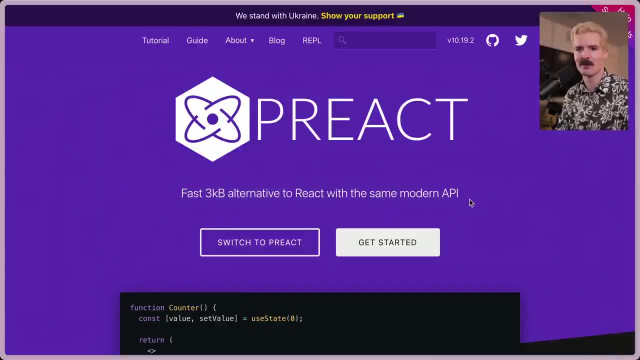 its focus is the bundle size, And they have some of the strictest bundle size rules of any project I've ever seen. If you want to add a new feature to pre act, you either have to build it externally as a library or delete as much code as you add in order to make sure it's bundle size doesn't go up. 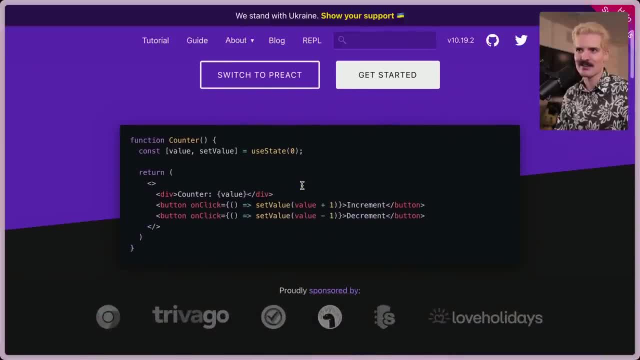 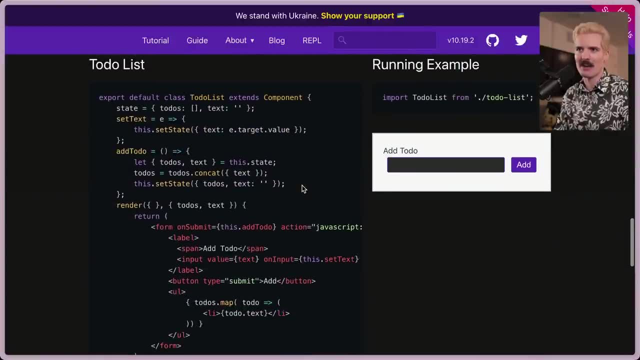 in the process Really really cool. It's not react, So you can't just like take a react project and expect it to work. But it does work pretty often And you can write a lot of the code you're used to writing with react in pre act, both with class. 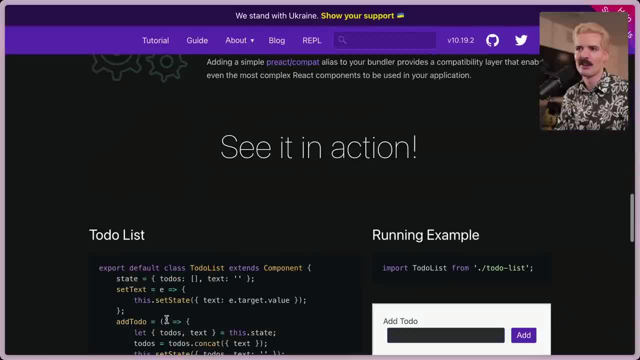 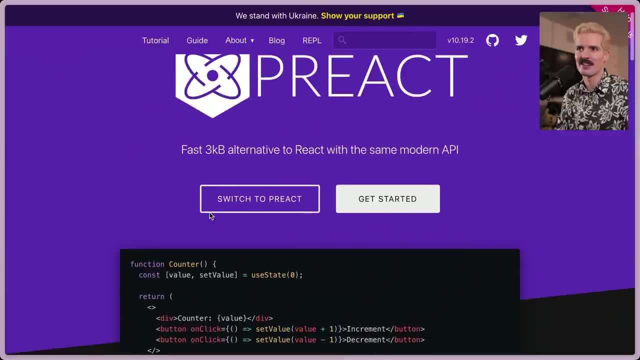 components and also hooks. They have the hook one on top here, But the rest is still class components. That's kind of hilarious. That's really funny actually. But yeah, react is cool. It's nice having an alternative to react like this. One of the many cool features. 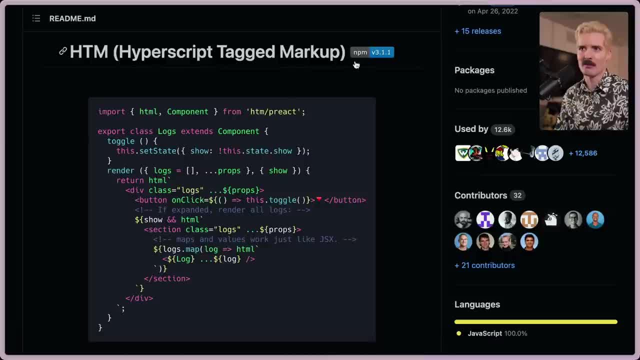 of pre act is HTM support, which is hyper script tag markup. It means you can use a template literal in JavaScript, which is when you put those little like back ticks after a function and it calls the function with this as a string input And by doing: 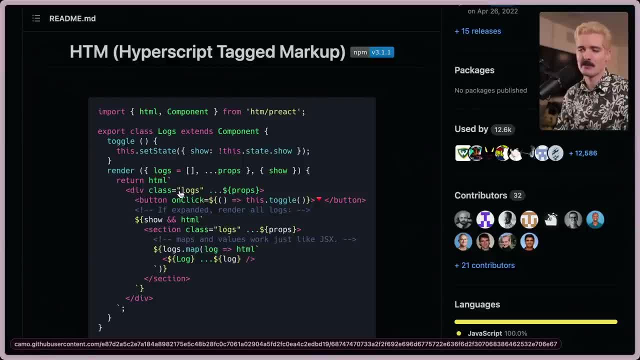 this, you're able to write effectively JSX inside of your JS, not need a transpilation step, And this gets parsed at runtime. So you can make a project that uses pre act in books and works the same way you would expect react to work, without needing a build step at all. This was actually a really 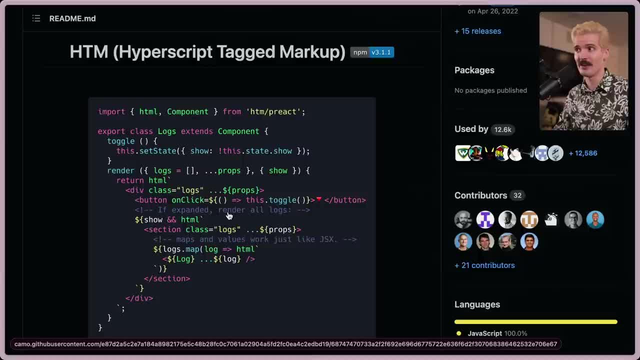 important framework for me as I was starting to deepen my understanding of these technologies, Because it helped me understand how all the parts assemble and not have the black box of the builder abstracting a lot of those parts from me. So I personally owe a lot to pre act. They also 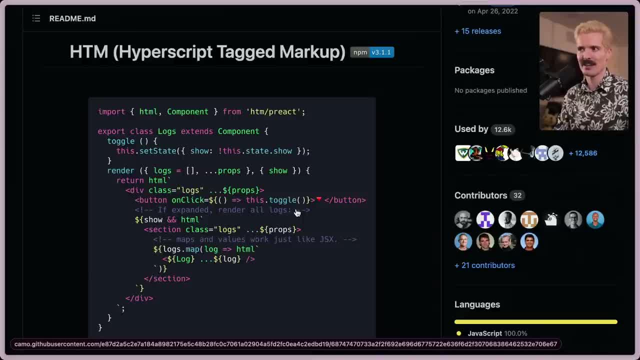 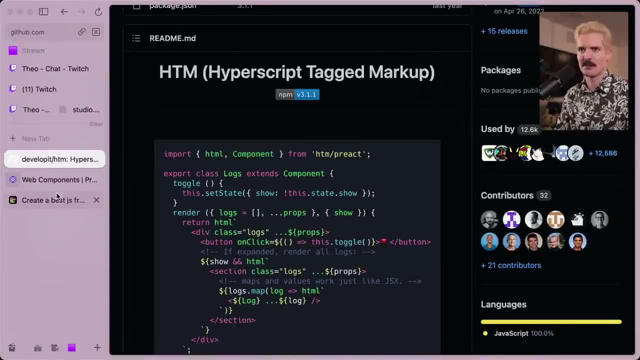 were the first to get signals working in react, which is really cool. to that all said, the recent numbers in the performance benchmarks haven't been as good as they used to be when comparing to react, which is obviously the framework it's built to compete with, But it's also 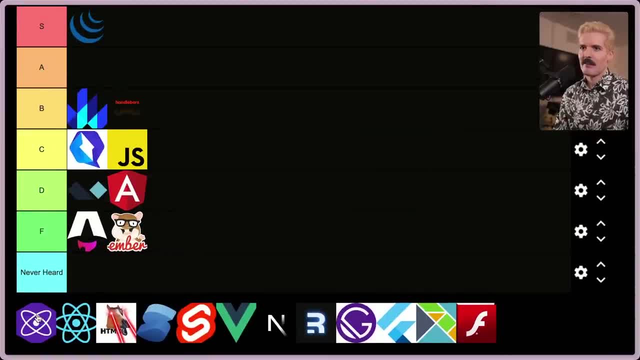 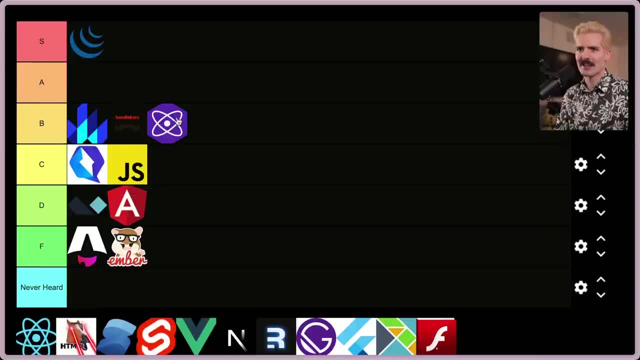 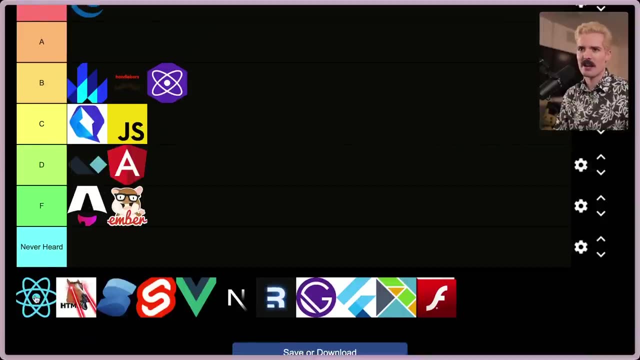 really important for the web And I'm really happy it exists. I feel bad just putting more and more things into B tier, but I'm doing it. beat here. Really good educational tool, really happy it exists, useful in certain use cases. not what I would reach for. Speaking of what I would reach for, we have now reached react. 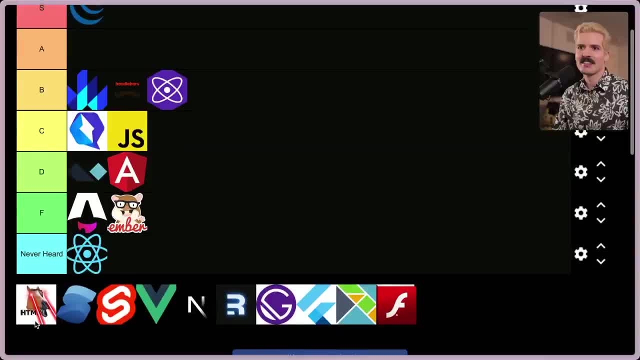 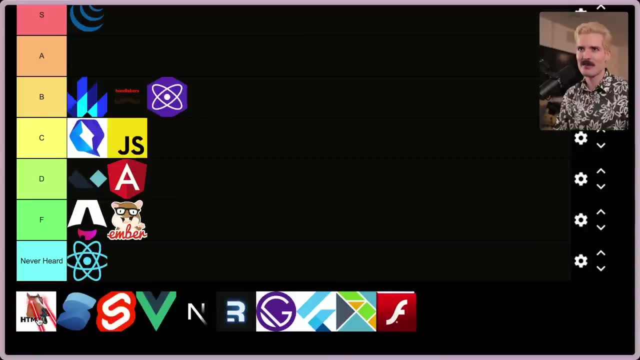 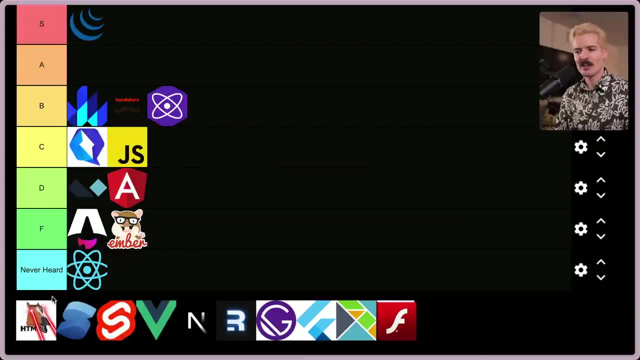 which obviously I've never heard of HTMX. HTMX is an incredible new framework that allows for non JavaScript developers and back end focus developers to make interactive web applications. If you've ever worked in traditional back end world trying to build a web app- usually the 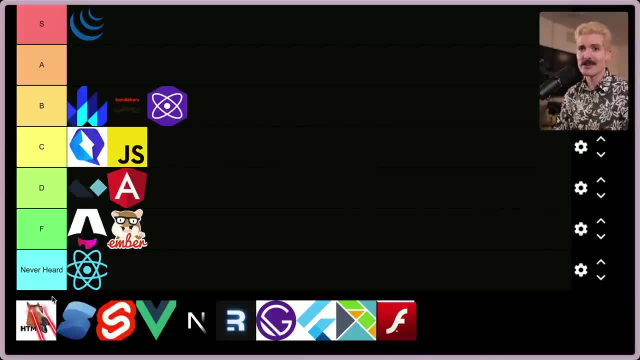 experience is, once the user has loaded the page, the only way you're going to build a web app is only way they get new data is if they refresh the page or if they go to a different route or if they post from a form. But if you want to have a button that has like a loading state when 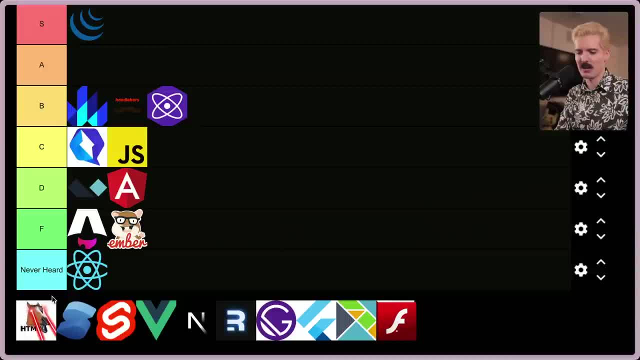 they click on it. or if you're trying to make a Twitter clone and you want to be able to type a new tweet, press enter and have the new tweet appear in your feed without reloading the whole page. Those types of behaviors were really hard to do without introducing a JavaScript framework. 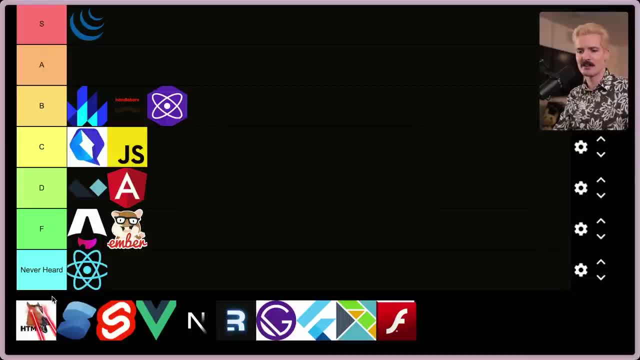 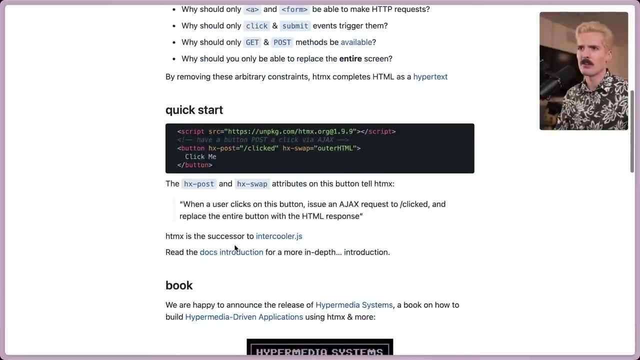 which is why HTMX wrote that JavaScript for you And now you can just bind to a template directly. I have a whole video about HTMX and why I think it's so cool, But I'll show you a bit of the syntax super quick. It's similar to what we were seeing before with Alpine, But here the 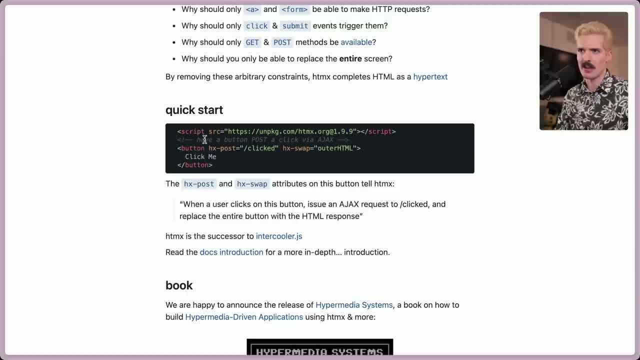 syntax is quite a bit more powerful and doesn't involve writing weird inline j s. HX post means when you click this button, it's going to post to this endpoint. slash clicked and HX swap outer HTML means whatever this responds with, that HTML content of this response is going to replace the. 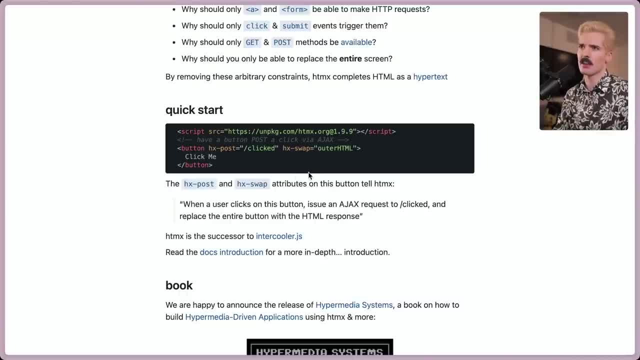 button. So if this returns something else, like a div that says thank you, then once you've clicked this and it's received that response, this will be replaced in your DOM with a div that says thank you. This allows you to do a lot of different things, For example, if you want to add a new 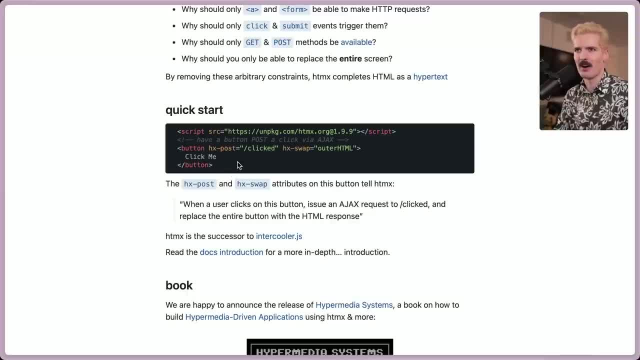 JavaScript. you can add a new JavaScript component to your DOM And this allows you to not have to write JavaScript or client side code at all, And just change your template up a little bit. in literally any existing backend framework, It can be JavaScript, it can be go, it can be rust. 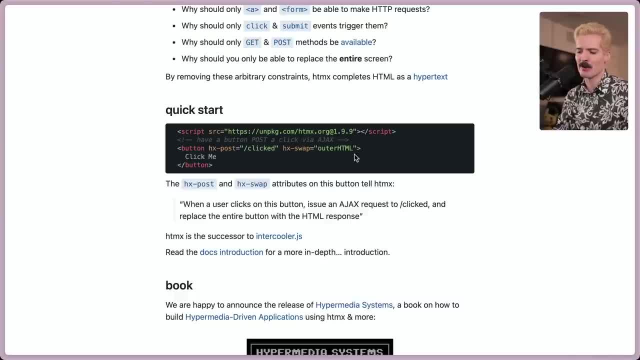 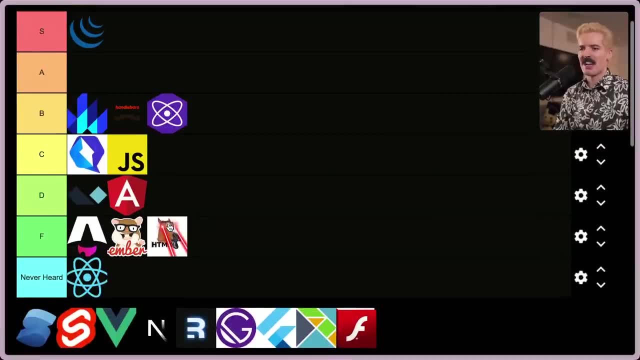 it can be Python, it can be Ruby, it can be anything, and just have better experiences for your users. For all of those reasons, I have to give HTMX an F tier because, again, it's not a JavaScript framework. Anyways, let's talk about solid. solid, first and foremost, starts with the 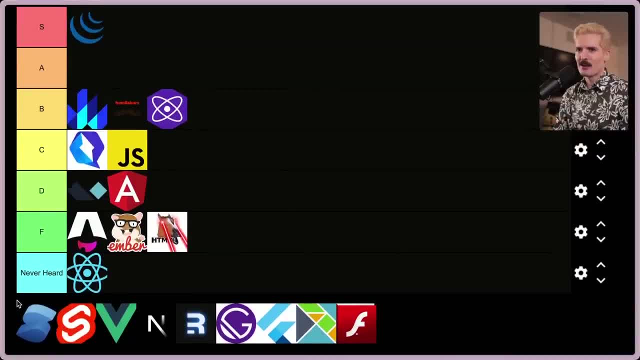 letter s, So I think you guys can guess where we're putting it. The main design goal of solid JS was to bring back the glory days of knockout and try to make something that made signals approachable and fun to develop with, while not compromising on performance at all. 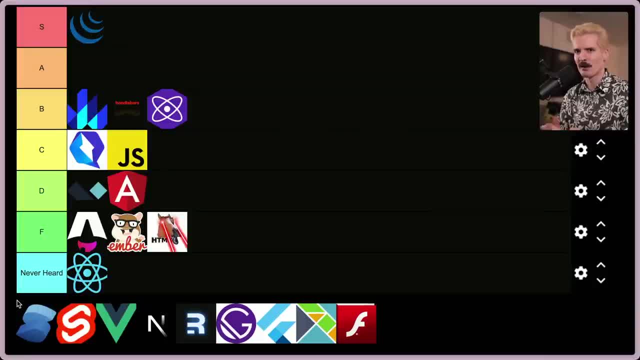 I still remember the first time I saw solid pop up in a benchmark and I was blown away because it looked just like react code, because it's still using JSX under the hood. It's still JSX when you write it, but it was performing almost as fast as vanilla JavaScript in every 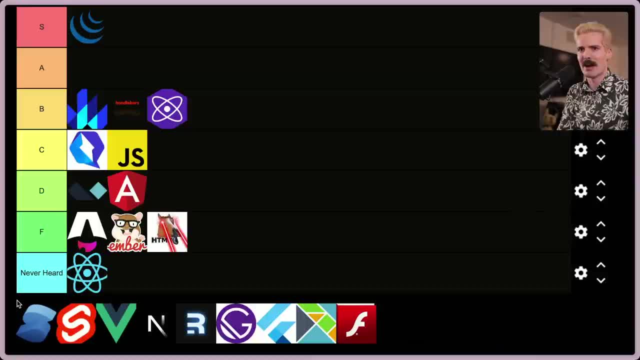 benchmark, I saw- And at that point I still believed- JSX was somehow causing performance issues And theoretically, if you wanted the fastest app, you wouldn't use JSX and solid prove that wasn't the case at all And this is one of the best getting started that we've seen. 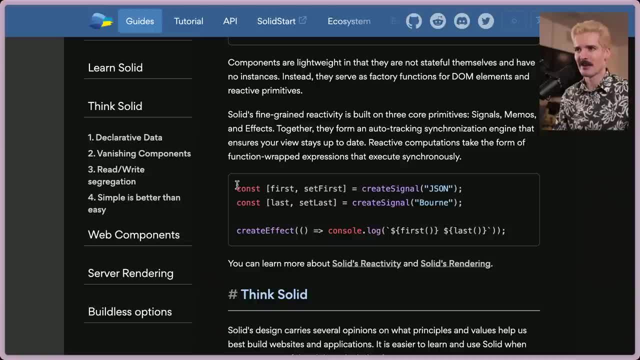 so far during this, It's immediately talking about the code that's specific to it. So first set first is create signal, last set last create signal. Think of this like a use state in default values and you can create an effect. The catch is when you use first and last, you're not just dropping. 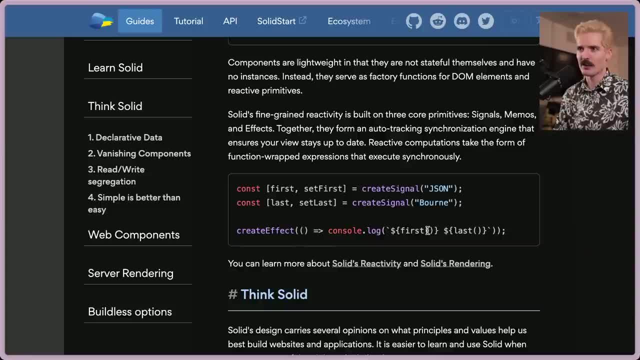 those as values. you're actually calling them. The reason we have these function calls is so bindings can be created through the signal layer. signal is an update chain where, when something changes, it knows everything that's going on. And that's what we're going to talk about today. So let's get started. 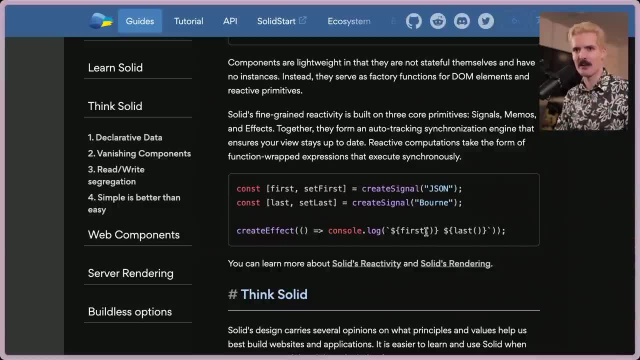 Everything that needs to be updated immediately. with react, it just changes everything from the top down with solid. since we called first and last in this effect, it knows when those change this effect has to run again. Here we have an HTM based vanilla JS example with solid so that you can just. 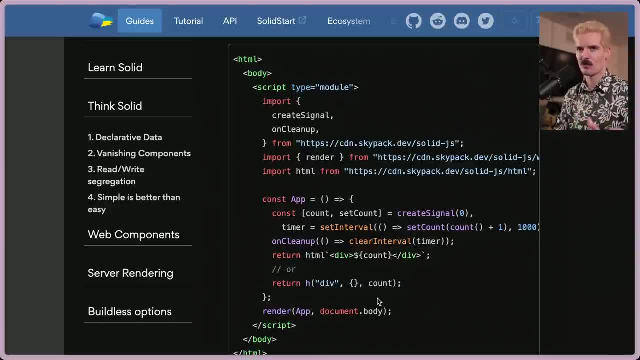 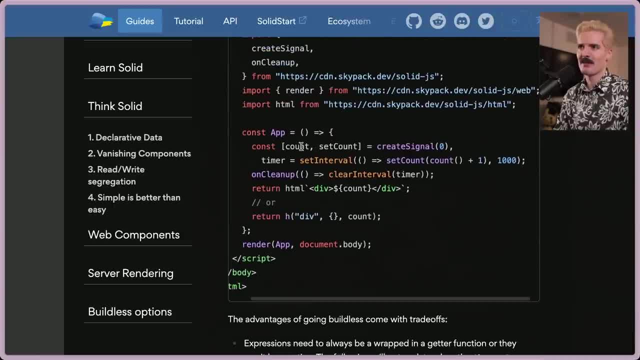 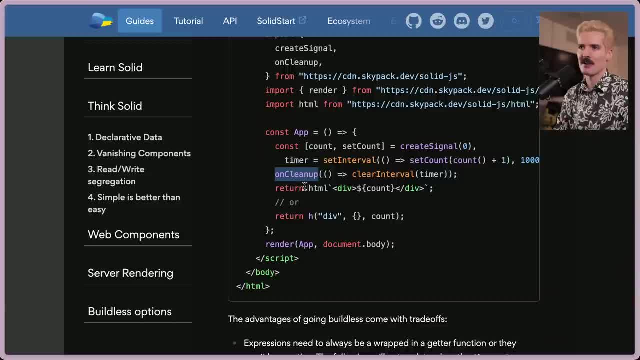 the count every second and on cleanup, you just call wherever inside of your component and now it will clean up and run this when the components goes away And you can return HTML or you can use H, which is very similar. This is kind of how old react code would render before JSX. This is: 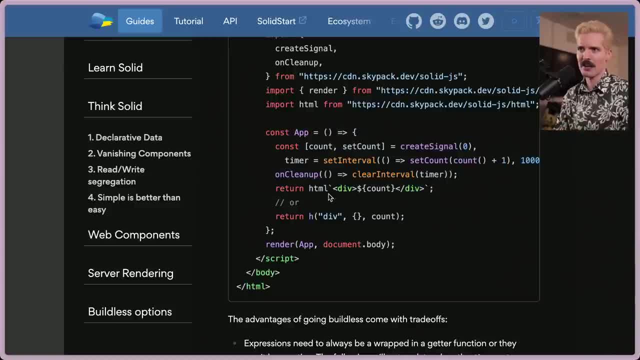 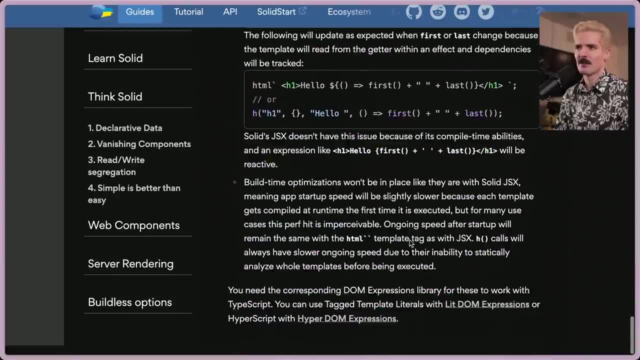 all you have to do in order to make a component that updates itself. You can also make it a button and bind the on click to update to in the same way you would expect. It all just kind of behaves how you would expect it to, which is really really cool. Solids, a great framework. solid start is. 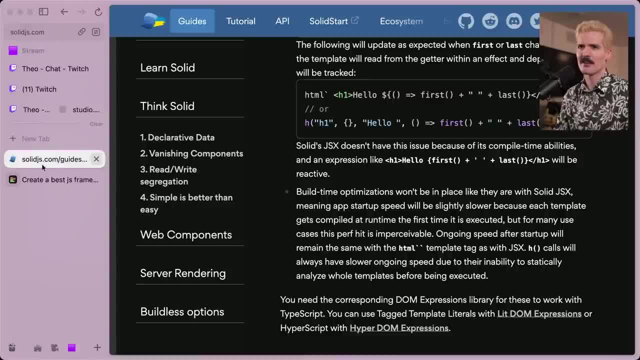 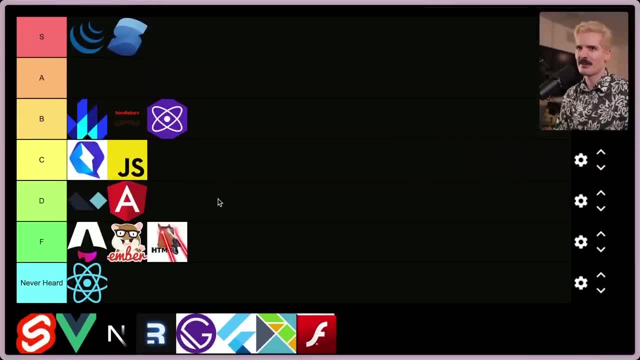 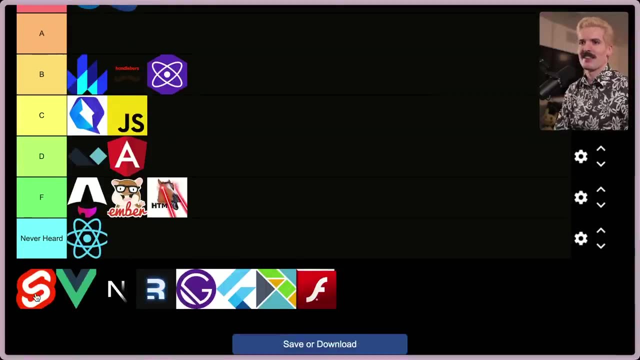 making a ton of progress as well. Do not discount this framework. I still think we've yet to see the deserved rise of solid. I'd put it just behind jQuery in s tier, And when you consider the fact that it's already got an s, that's two s's for solid Heartbeat. Speaking of the letter s, 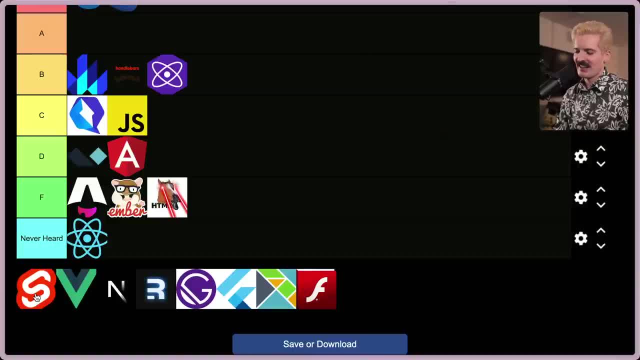 we have svelte. How does one talk about svelte? It felt was a very important framework for me because it was the first one to really challenge my, my diehard react bro nature. I remember the first time I saw rethinking reactivity by Rich. 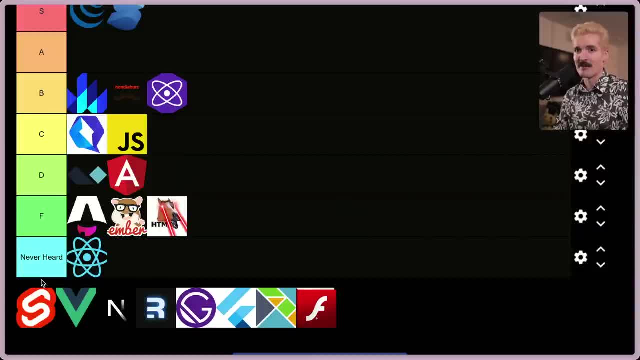 Harris Phenomenal talk. I have a video all about my favorite tech talks coming soon. Subscribe if you haven't, by the way, because then you'll get to see that video right when it drops And come on, subscriptions are free, guys, helps us out a ton. Anyways, svelte, This framework showed me that. 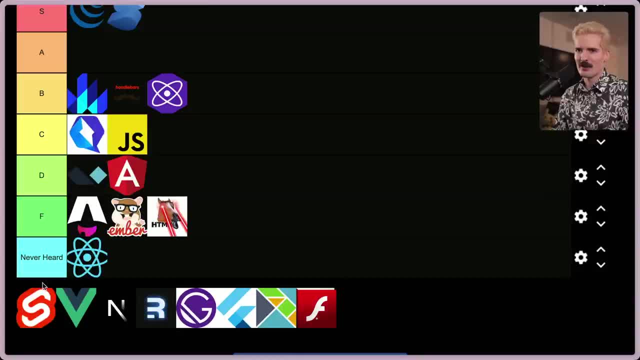 first off, react wasn't truly reactive But, more importantly, it showed me there were things react didn't do that made my web development. It showed me that React wasn't truly reactive But, more importantly, it showed me there were things react didn't do that made my web development. 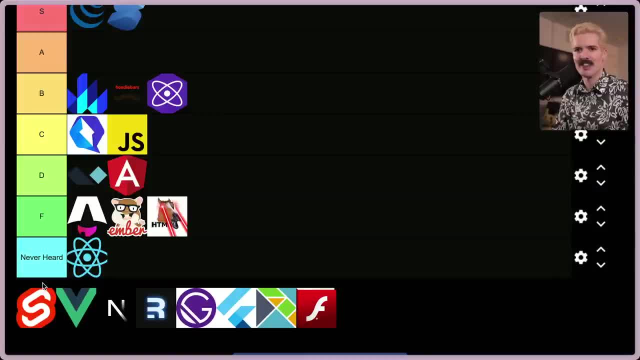 experience a bit more painful, like react had no opinion on styles And that started to really hurt once we got into react native, where they had to have an opinion. react doesn't really have an opinion on builders or bundling. Now it kind of has to because they moved to this new server. 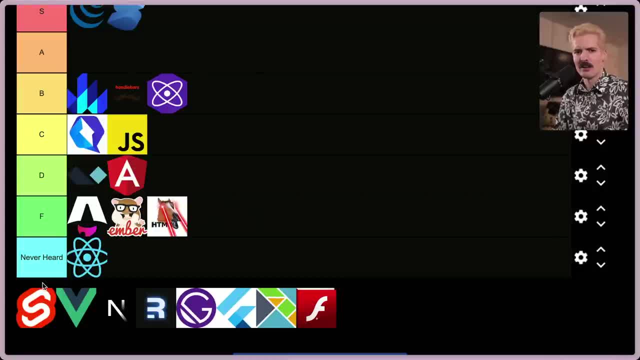 component model, But previously it didn't at all. Now they just throw out a webpack plugin and partner with the next team in hopes of figuring those things out. svelte's done a lot That's really good, like a lot, But they also have done a lot of things that I personally don't love. 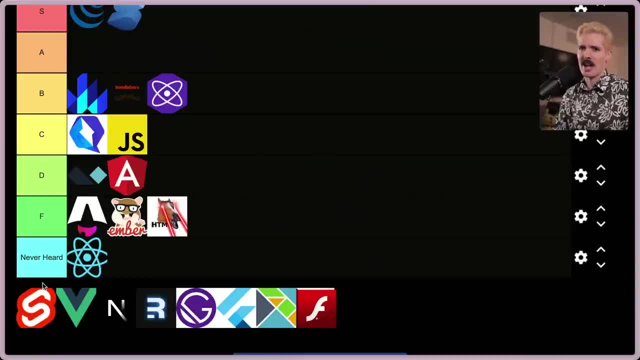 The big one for me is single file components. When I'm working on an app and I have some piece that I want to reuse, I want the ability to break it out quickly and not have to lose the context of the file that I'm in. This is a problem I have with view as well, So we'll talk about it more. 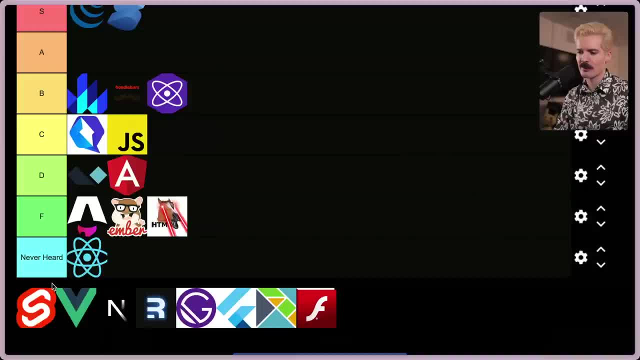 there. By using svelte, you have now committed to a specific code architecture that you don't really have control of because of the way svelte is designed, And I know a lot of people really like that, because it means all of the components are going to have everything contained within. 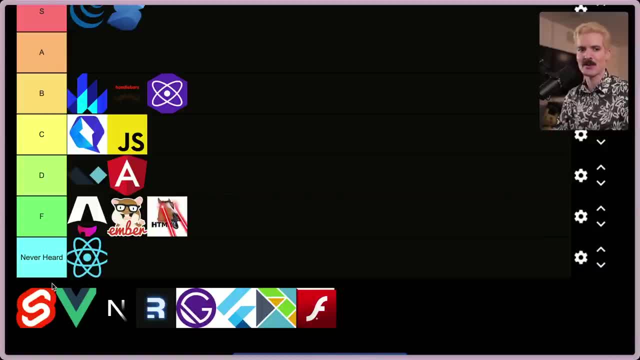 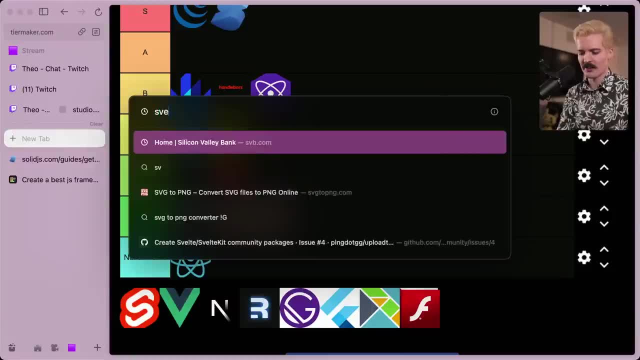 them. But it also means you have to do crazy things with your markup syntax, And this is why in both svelte and view, we see a lot of weirdness in their templating. Neither of them are using JSX And in svelte you're using svelte's weird markup syntax. Sure, they have some good examples. 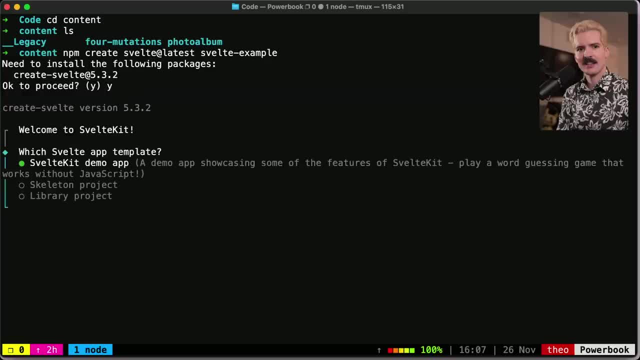 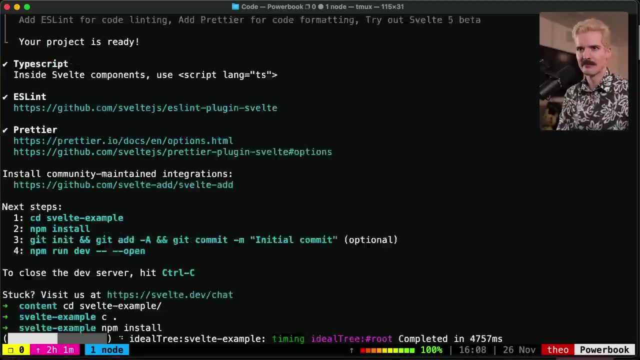 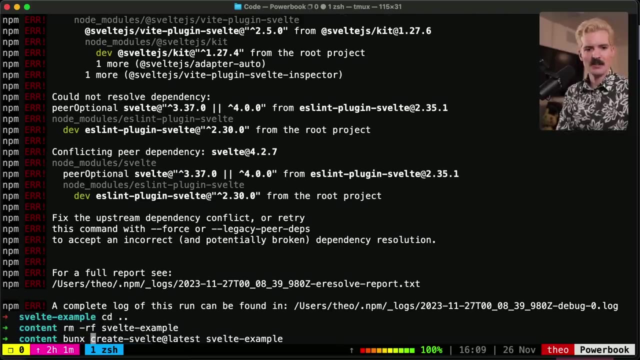 Do they have the like getting started? Cool, Get this started quick. svelte demo app: TypeScript. I don't like the default to the JS doc. Now do I try out svelte five? I kind of want to try out svelte five. Good start. Let's not do the svelte five beta and do something risky, Okay, cool. 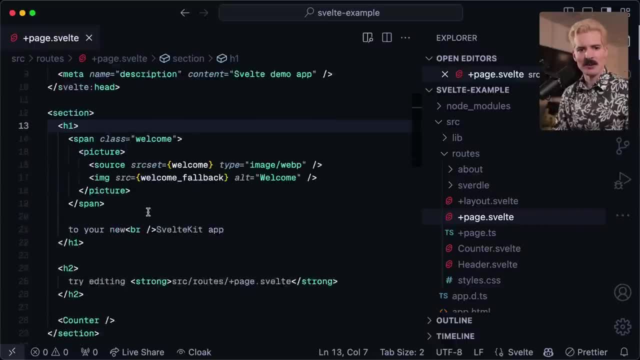 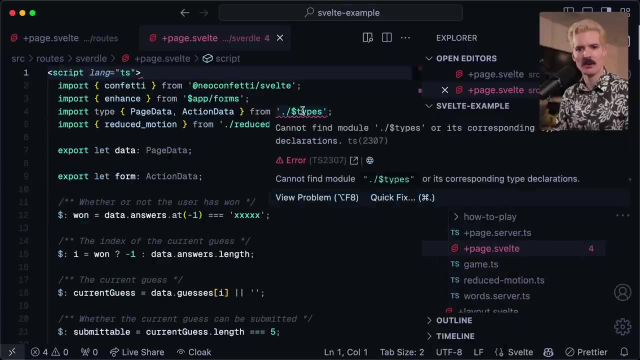 Stop complaining, Nice. It's just the. the recent beta seems to be broken. Anyways, this is a default page. Not much interesting here. svelte is where things get interesting. This is their Wordle clone, And apparently you have to run bun dev once just to get your type. 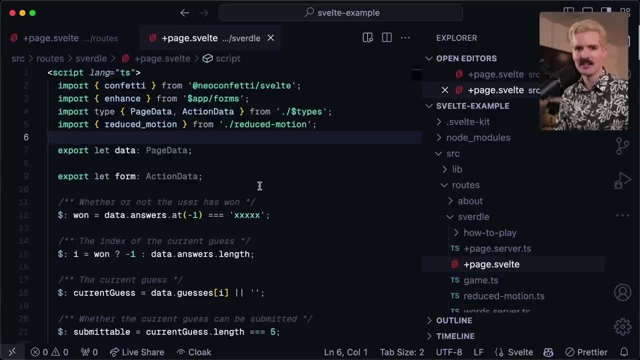 definitions, because they generate those via the dev server, which is again one of the problems you run into when you're not using vanilla TypeScript, because they have both their custom template syntax and they have implicit behaviors like let data page data this binding and these: 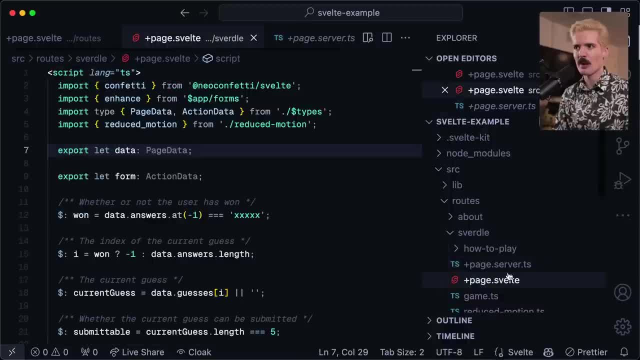 definitions. these come from page server TS, but we're not importing page server TS. We're not importing. We're importing from dot slash, dollar types, which is a generated file that gets created and hidden by VS code once you run the dev server, such that when things change here, it will get. 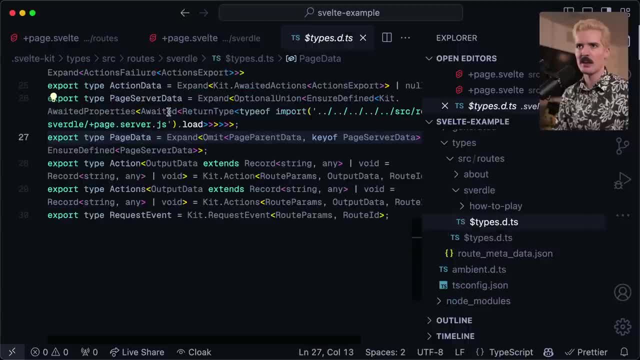 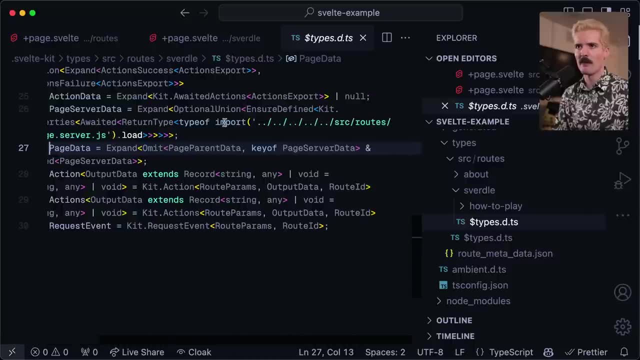 updated accordingly. Thank you, even go to the definition. Yeah, And you can see. it is this crazy: generated types, DTS stuff, But thankfully it is actually generating the type directly off of the page server JS file, So you don't have to worry about the type definition being stale if you close. 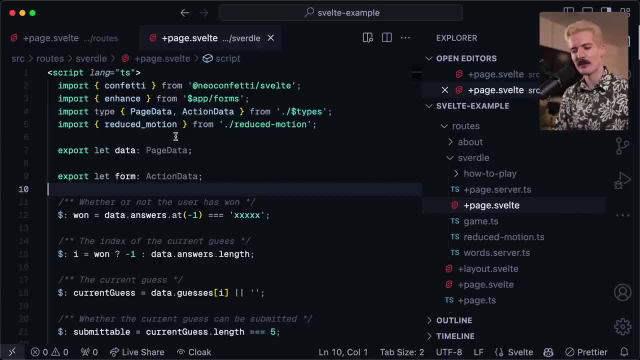 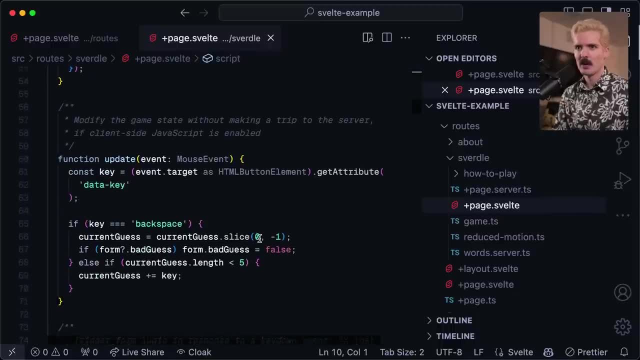 your dev server. Yeah, not great. This is why I like something like the new server component model where you can just await in the component. But that's not what I'm here to talk about, And I know they're working hard on continuing to improve the experience here. What I'm here to talk about. 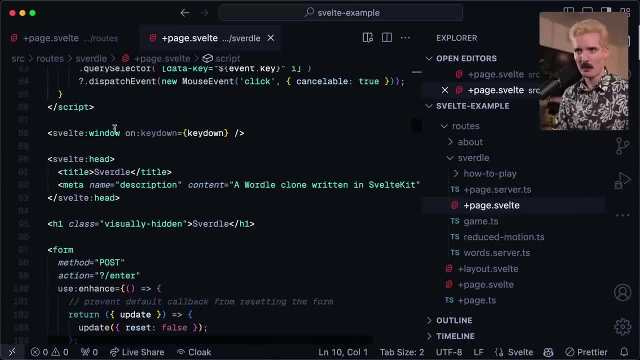 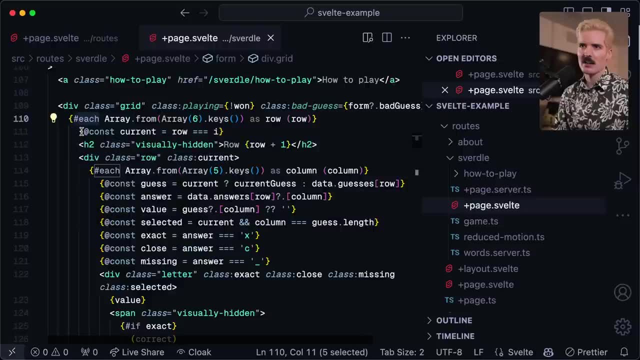 is more of the weird syntax decisions Because we have svelte colon window, svelte colon head, weird but fine. But here's where things start to get a little weirder. Hashtag each at const: current equals row, equals, equals, equals I. that's not how JavaScript works at const. What is this? 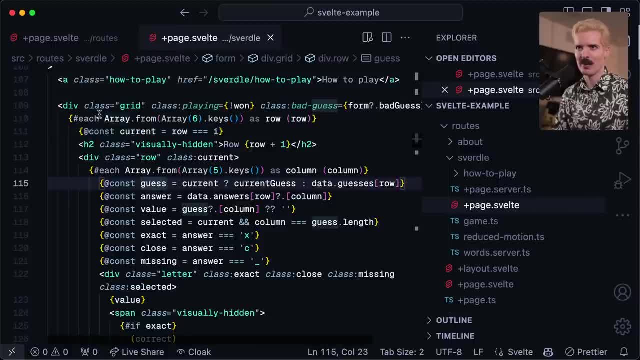 Well, because they built their own templating system and sometimes those templates need to be dynamic. they also had to reinvent JavaScript. in the same way that JSX is reinventing some of HTML in JS, svelte is reinventing JS inside of HTML here, And I personally don't love that. 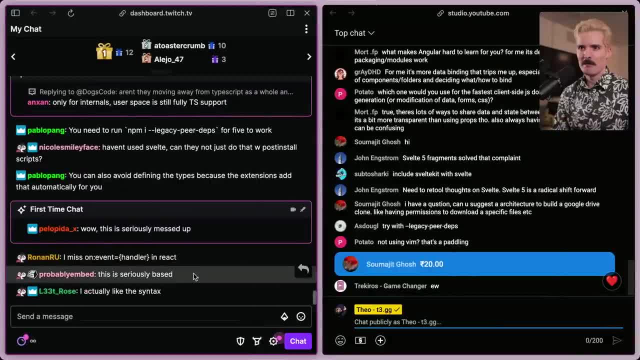 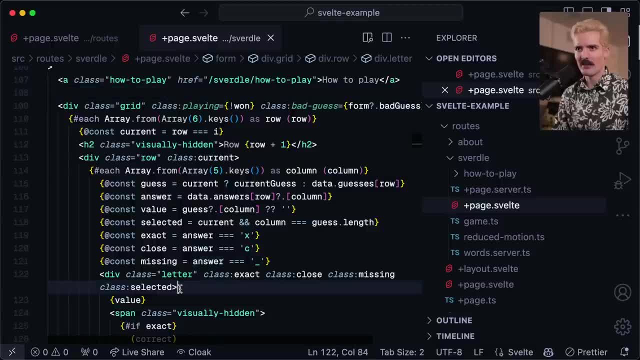 There's a lot of people who are going to. I already see embed in chat And, by the way, embed is based. they're the one who made this tier list for us in the first place And we're seeing people say they actually like the syntax. But I like JSX. I like that. my JavaScript is. 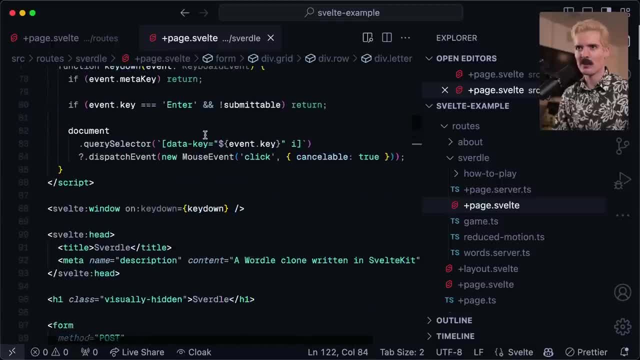 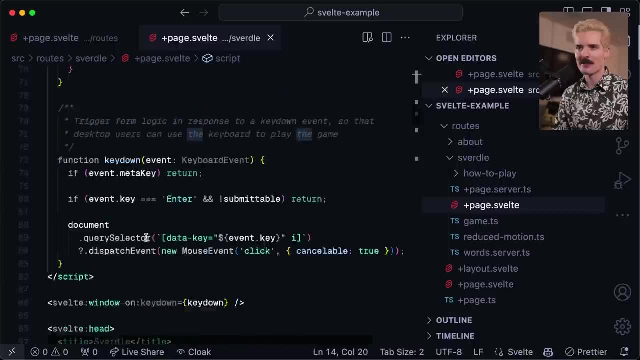 JavaScript and that I'm not writing a different JavaScript. once I've gotten below the line, Like in the script tag, you're still writing JavaScript will type scripts. you specify langs, ts, But from there down, once we get into here, once you're in your markup, 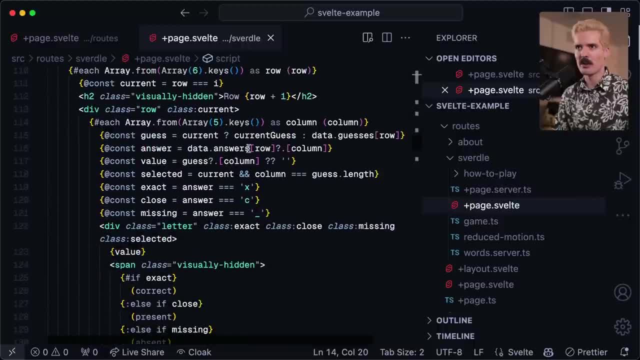 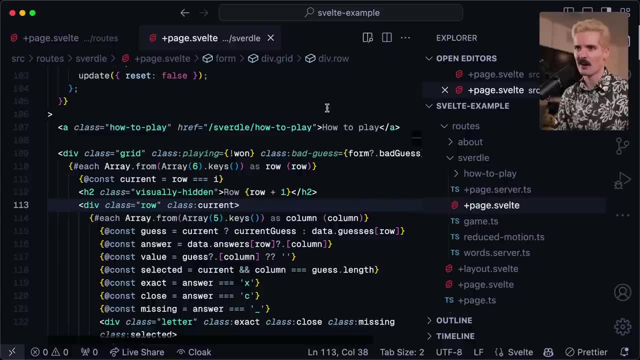 and you want to do things dynamically. all of a sudden you're writing this weird hybrid thing: array dot from array six dot keys as row parens row, like what you are saying in chat. it's hard to believe that anyone would call this more readable than JSX, Because 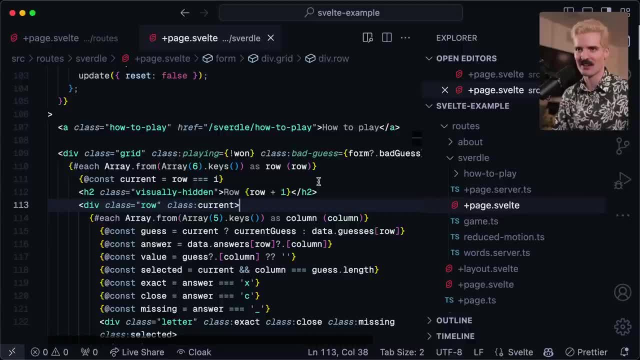 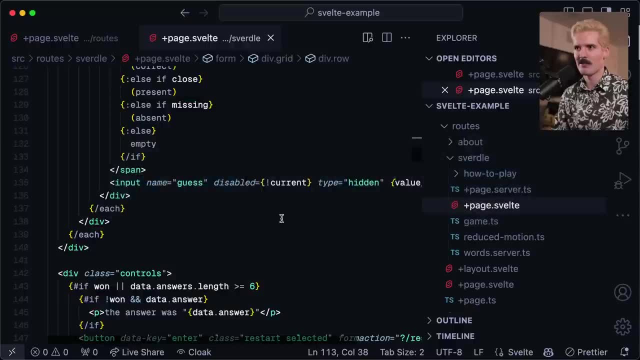 you just write the JavaScript for each or map in JavaScript. It's weird. I will also give credit to svelte devs. it seems like a lot of them don't use this type of thing But at the same time, this is the example that you get when you generate a new svelte app. So I'm not like 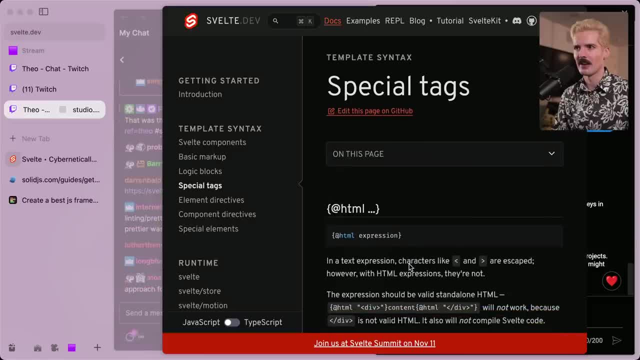 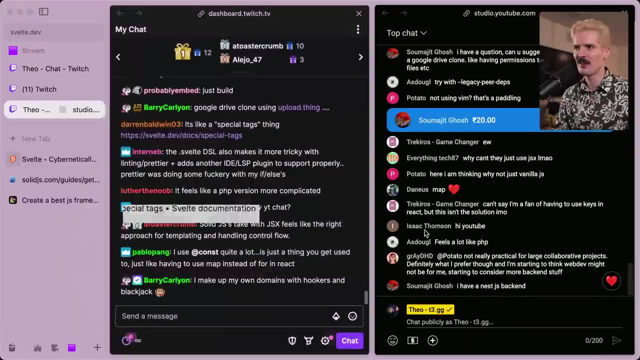 reaching really far to find bad svelte code. just is how it is. Oh yeah, they have a whole special tag section for svelte joy. They even have an alternative to console log at debug. It's cool They have that, but weird that you need that. You know what? I'm going to make some changes. I'm 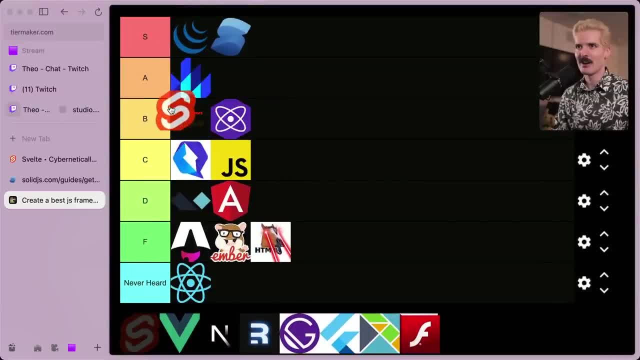 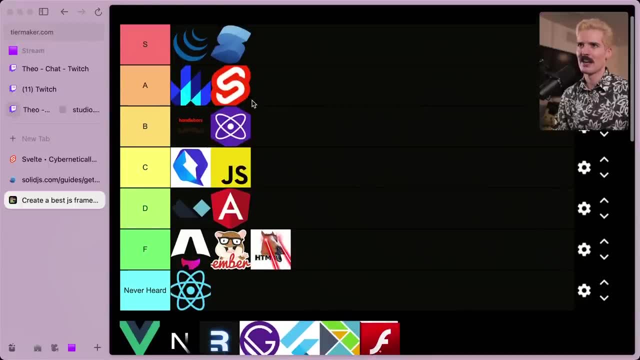 going to move lit up to a tier so that I can put svelte brunt on B tier. You know what I can do, that I can deal with, that I would. these are very close for me where, like svelte, so important. 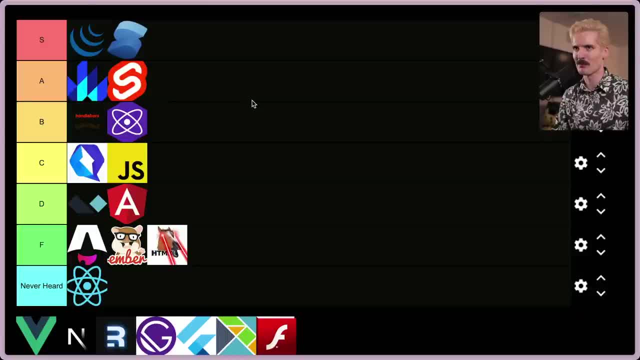 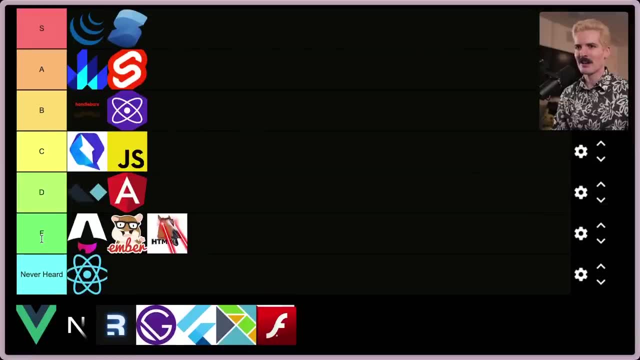 and it's pushing the right things forward. I love rich Harris. I think he's one of the smartest people in the space, But I wouldn't use svelte because I don't like the syntax. That's why this is tough for me Now that we've talked about a framework that reinvented the syntax for writing. 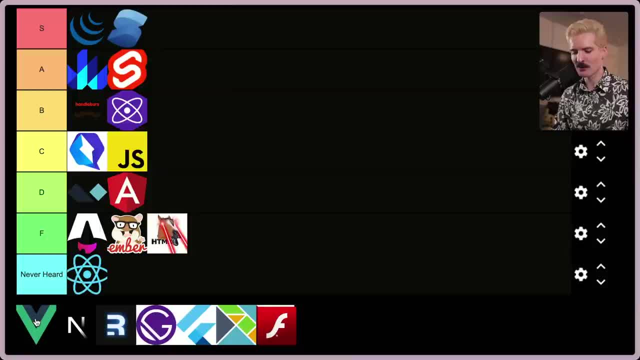 the code. Let's talk about view. View is really important And view has one unique characteristic that I want to go out of my way to call out. It's been misunderstood when I previously tried to do this. I want to be very clear. views international community is unmatched. They're. 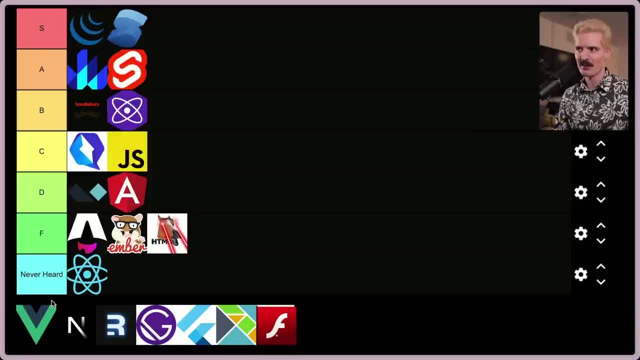 docs are internationalized almost as soon as they drop. There is so many incredible people all over the world working on view. The community is unlike any other community I've seen in the web dev world. It truly feels like everyone is able to join that community and take part in it. 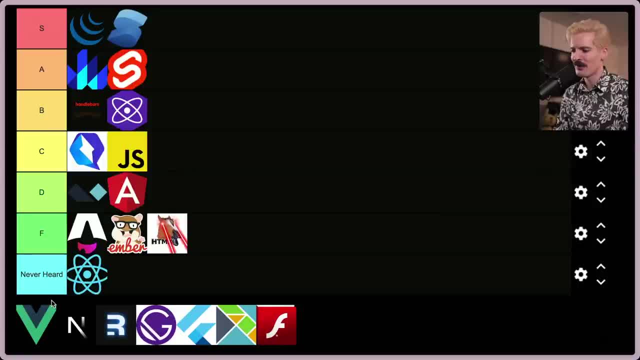 And that's a huge part of why something like V has found the success it has as well. The view community is incredible, And if English isn't your first language, there's a very high percentage chance you started with view, And I think that's an awesome win. I wish more of these frameworks. 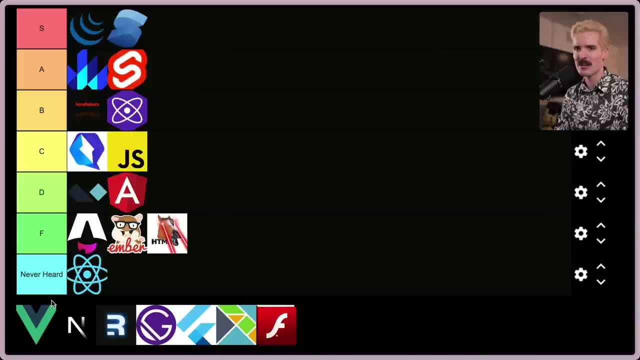 had communities that big outside of the US and outside of English speaking Western nations. That said, they kind of started the single file component trend where they made the dot view templating syntax and they kind of require you to keep everything in those files And if you want to, 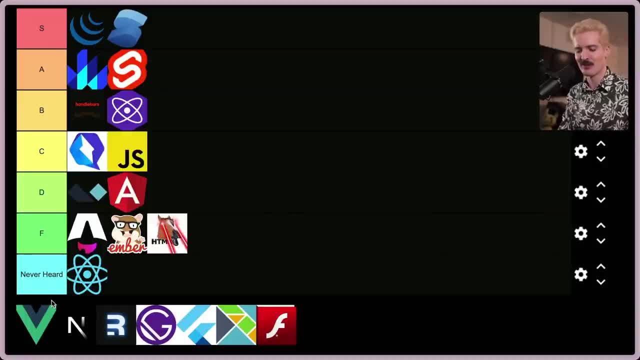 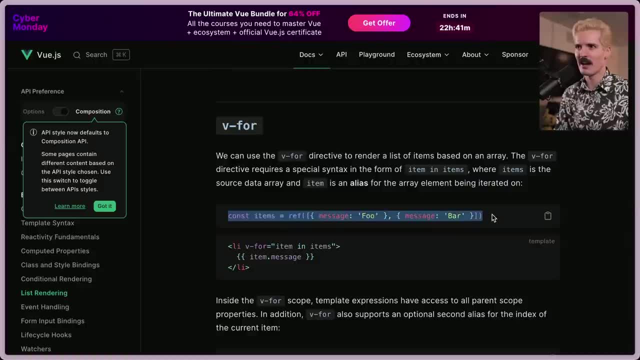 break out a little bit of logic to reuse, you end up with a lot of the same problems I just showed with Svelte, Similar to what we just saw with Svelte. they have a four equivalent, but for them you define a ref with items or whatever you want, And then you have this V dash four syntax. 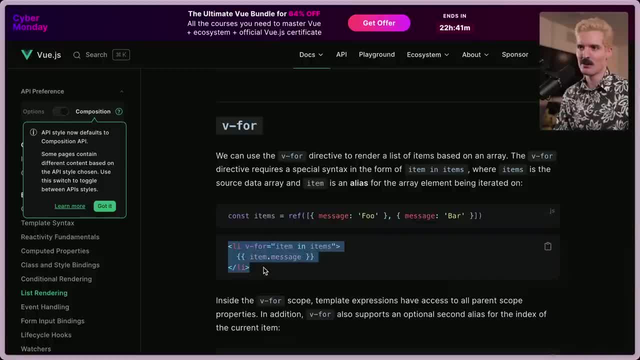 which specifically tells the view runtime to make a new one of these components for each item in the list. it kind of requires you to do more of the work outside of the markup and inside of the JavaScript layer, which is nice, But it also means that things you can do in it are inherently less. 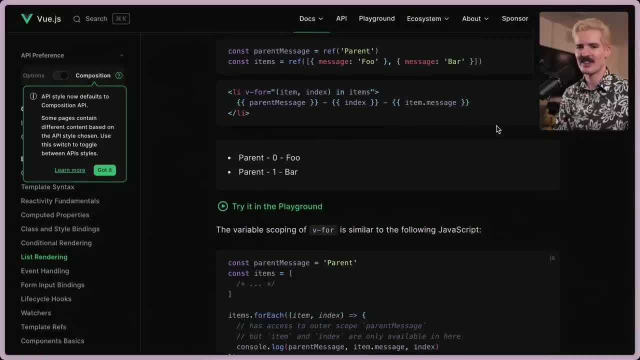 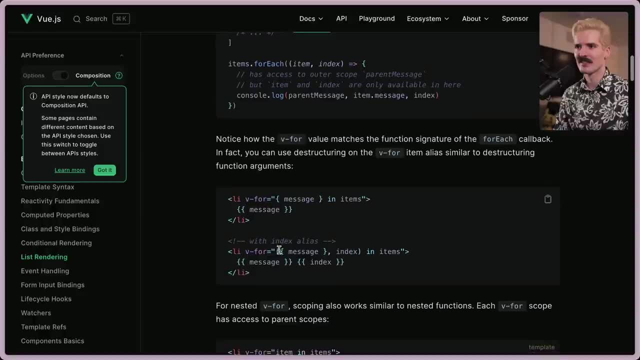 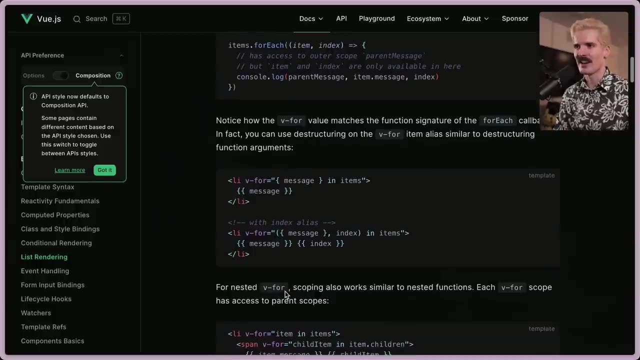 dynamic as a result. So it's checks and balances, you know items, that for each item variable scoping is similar. And again it has this weird syntax for, like, defining a value. So it just takes a bunch of different JavaScript and then it just sets it up in line so that it has 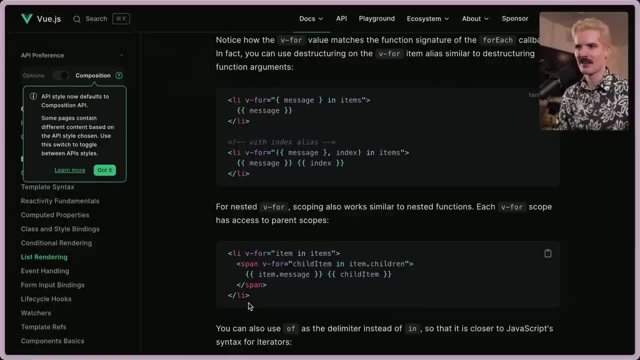 closures in scope, And now you have to learn about these specific behaviors. They're less mind boggling than the ones in Svelte, but they're still not just JavaScript, And I think when React calls itself just JavaScript and everybody freaks out, this is specifically what they're talking. 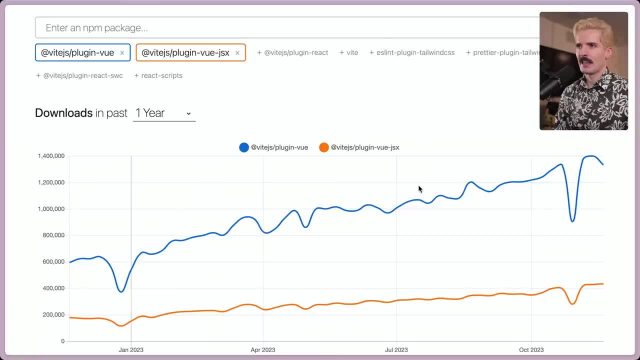 about- And yes, I know Vue JSX is a thing, But I want to show you guys something, because I have been hearing about this forever. That is not an argument: more adoption, but for less than one in three of the users to be using jsx when they're using view. 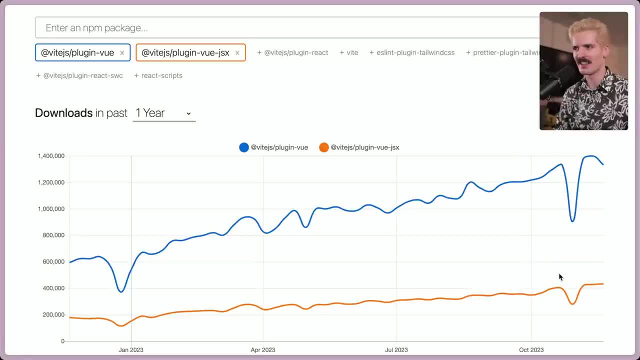 this is telling. this is very telling and i don't think view jsx is a good enough argument when it's not the standard and also from what i've heard on every release of view, it tends to break and you have to wait a while for it to catch up- similar to the next experience that all said. 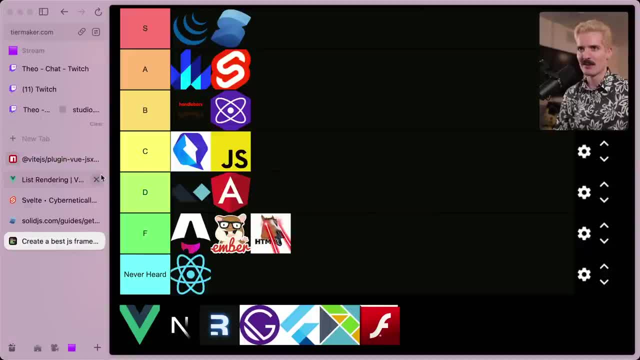 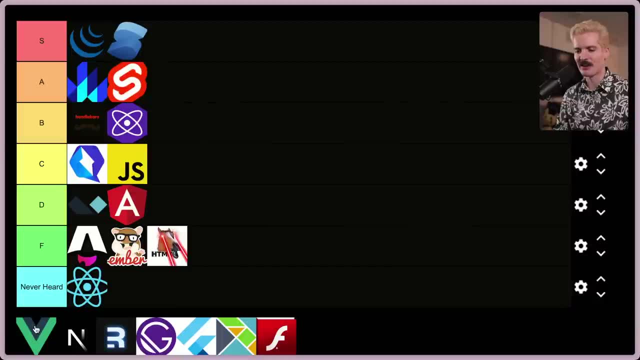 view is still very, very good. there's a lot of people i know and trust who still lean on view as their go-to- and i think that is a very good choice- and a lot of teams, especially those that aren't primarily native english speakers. the state of the view community is just so much better. 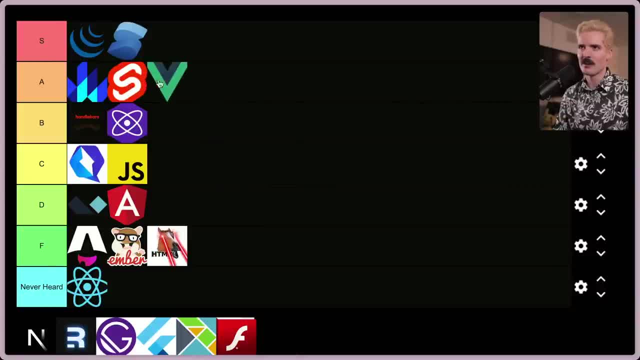 that it it deserves a low a tier. i still would use felt first and also view needs to ship vapor already. if you're not already familiar, view vapor is their attempt to rewrite view such that your code doesn't have to change, but under the hood it's running very similar to solid. that's why 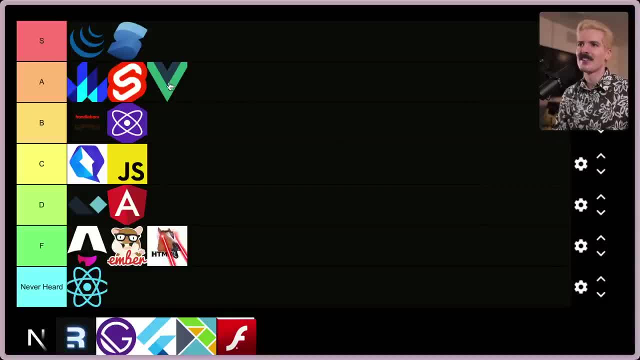 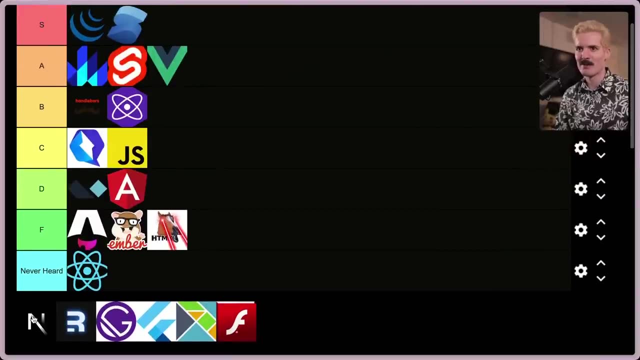 it's named vapor. it's a pun on solid and like states of gases, so very excited for vapor if that can actually happen. view, not a bad choice. love the community, don't love the syntax, don't like single file components. let's talk about next, oh, next. my issue with next is that most of the things that compose next and that are: 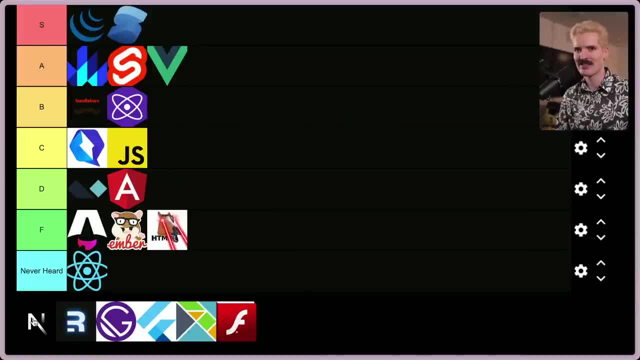 truly unique to next. i hate, especially from the pages era god, i hate to get server side props. it was the wrong way to do server side data. it was an attempt and it was a really bad one and i i didn't enjoy it. that said, it was one of the best ways to build backend integrations for your front. 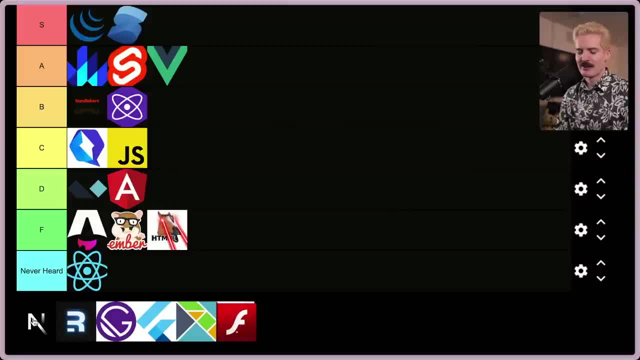 end app but almost all of the the front end code in the original next versions pre-app router was based routing you got it. wasn't worth it but for the api directory where you could quickly serve json payloads from an endpoint inside of your react app. with good relationships between those. 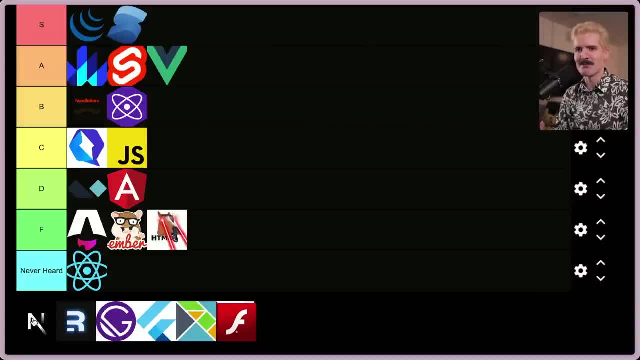 if you use something like trpc. next, js's primitives were in an incredible state to be abused and i abused the hell out of them. so for me next is an s? tier for what you can do to it, but its actual core pieces were f? tier. now i'd put them at a solid b i had with the new model. there are many. 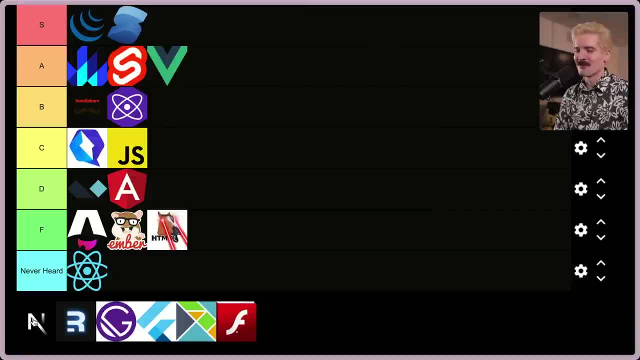 more primitives that are very fun to play with and i've been doing some nonsense with those, some pretty absurd shit. but man, i i find a lot of the decisions bad still. i have a whole review of app router where i talk more about this, but i'm i'm just still not that into file based routing. i get why they do it. it. 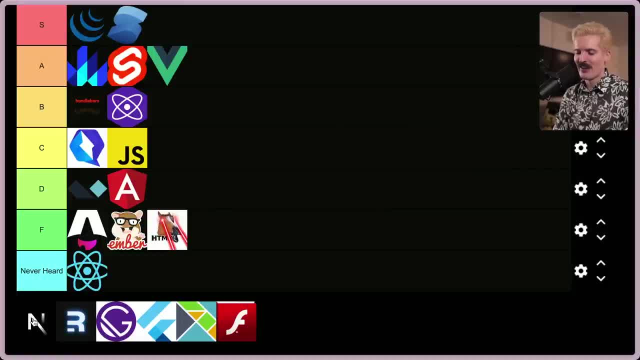 makes the compiler easier and it makes onboarding in a code base easier. but overall i feel like most of my recent love for next comes from server components, not next, and for that reason, hi b tier, let's talk about remix. i have talked about remix a lot and i will say i'm much more hopeful for it. 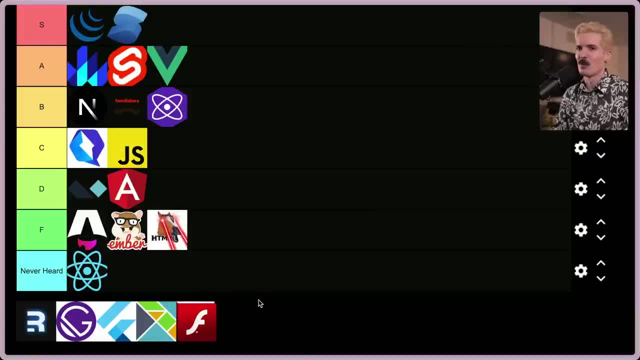 now, recently, mark dalgish has joined the remix team and he has been doing wonders for them- the best i've seen it, and it's going really far, really fast, while it doesn't seem like they're prioritizing server components, which kind of sucks, because i was excited for a more minimal server. 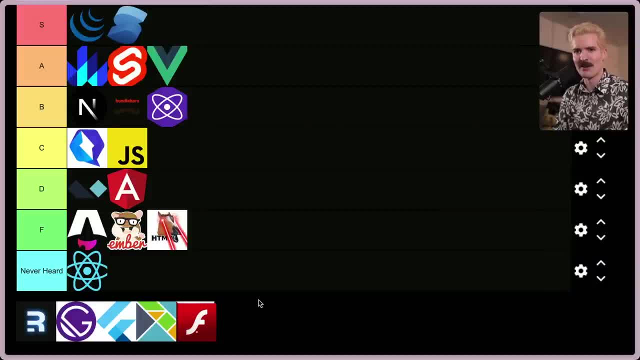 component implementation. they are getting beat working and that's what mark's primary focus since he joined. i'm really excited to see where remix goes with these new contributors, because everything i've seen for the past few months has been super exciting. that said, i still hate a lot of the 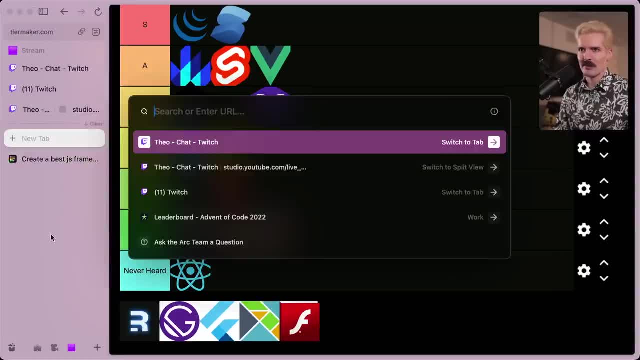 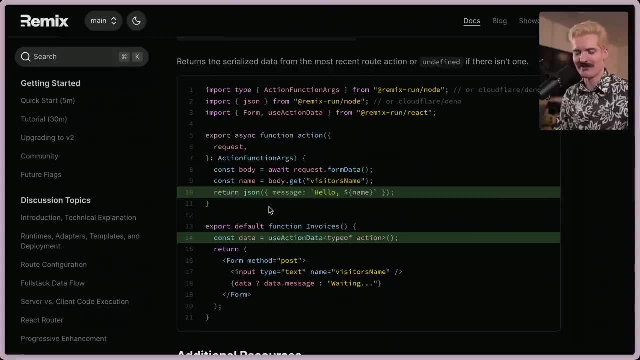 design decisions around remix. my favorite is when they show examples of how great use action is. so here's a basic use action example. an action is similar to a server action in next, if you're familiar with that, but in more generic terms, it's an endpoint that you can post. 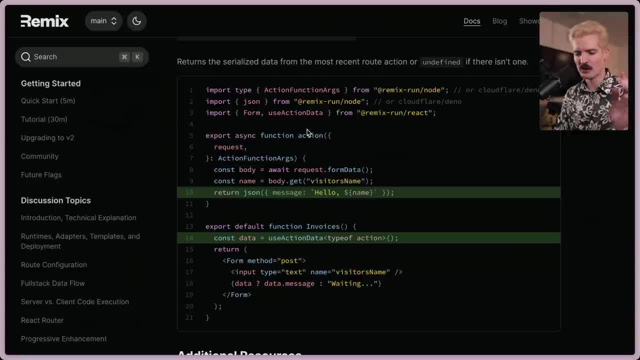 to. so when you create a route in remix, it can have one loader, which is what loads the data for that route. it can have one action, which is what happens if you post that endpoint. so if i want to post this action, i have to have a form that's on the same route. it just by putting the form in the same. 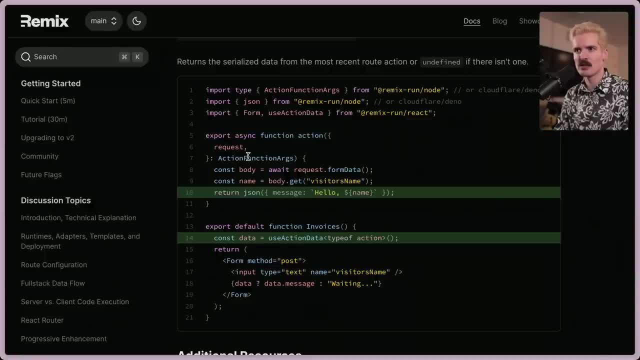 route, it will now know to post to this endpoint. but that means there's no relationship between these. like if i move this invoices component somewhere else, this whole model just breaks immediately, because it is required that you co-locate the code or you now have to deal with this crazy dependency chain. so if you have a component, 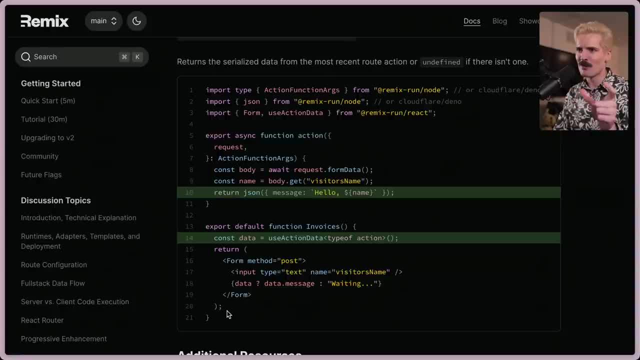 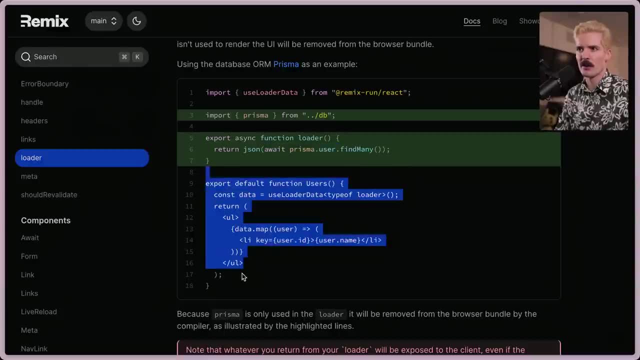 that needs some data and it's not in the page route. you better hope that that data exists wherever that component is mounted. so let's say you have this loader that grabs prismauserfindmany and this user's component isn't a page component. this is just in a different file. but then you call. 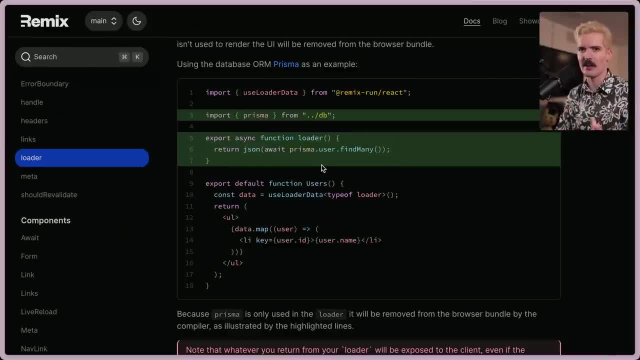 this in a route that doesn't have this loader. it just silently fails. and that's the problem when you have this route level separation, where you have a magic loader or action function that isn't actually being called from your network and you're just going to have to do this again and again and 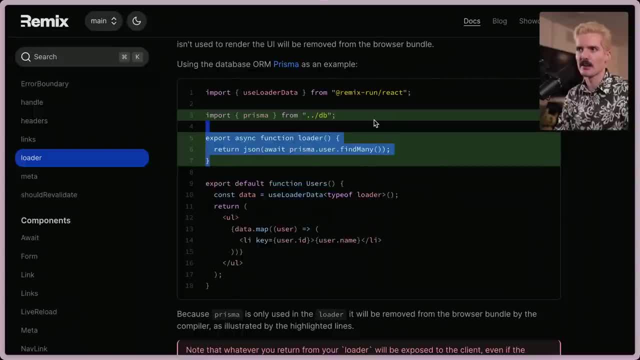 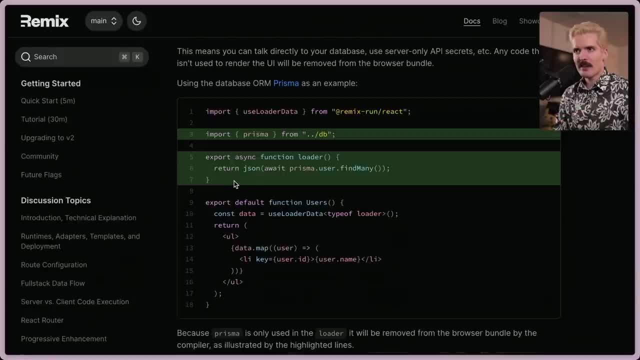 data and god forbid. you have a page that you want to post two things to. let's say, we have an action here for adding a new user, but we also have an action for deleting a user. now that you have that, you need to go define new endpoints or, even better, have a switch statement in your action that checks. 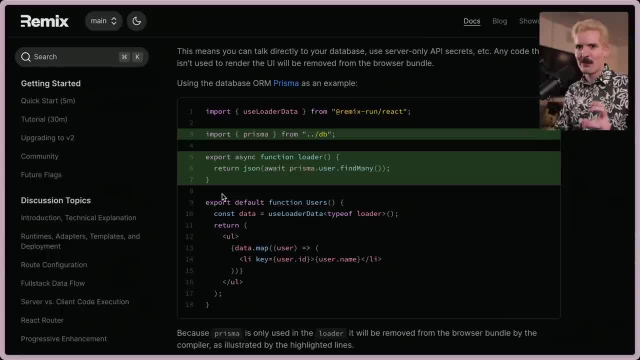 what type of action you want to actually do. so you're not writing an endpoint unique to the action the user does. when you define an action remix, you're not defining it for a component, you're defining it for a route and you hope that relationship between the route and the component. 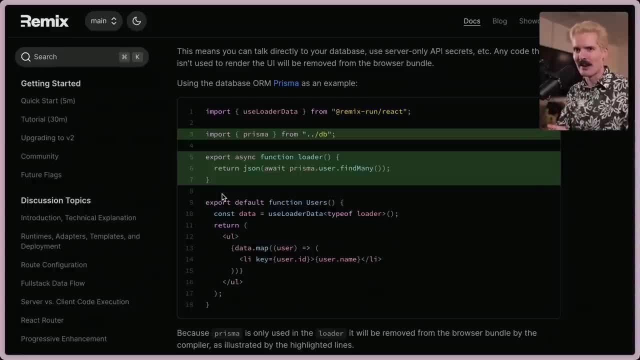 stays tightly knit and, as a result, i find it very, very rare that the action primitive actually ends up making sense. unless you have a code base that only one person is working in. it is just not a good primitive. for these reasons, and without a solution like trpc or an abstraction that 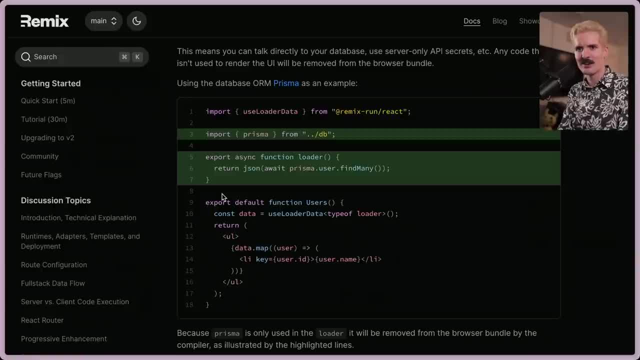 guarantees that one-to-one relationship, the same type of action you want to actually do. so you're not going to be able to do that. you're not going to be able to do that. you're not going to be able to do that. and this is in contrast to how things work in something like server component model with 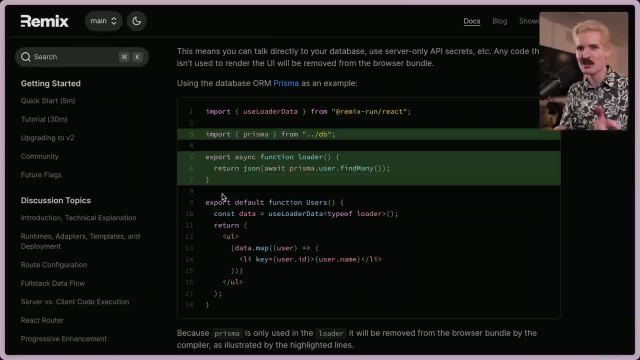 server actions, where you're actually importing the code, you're actually attaching the form to that definition and rather than having a big switch statement where you manually make sure each input goes to the right place, it just does it for you, and i don't like these non-deterministic. 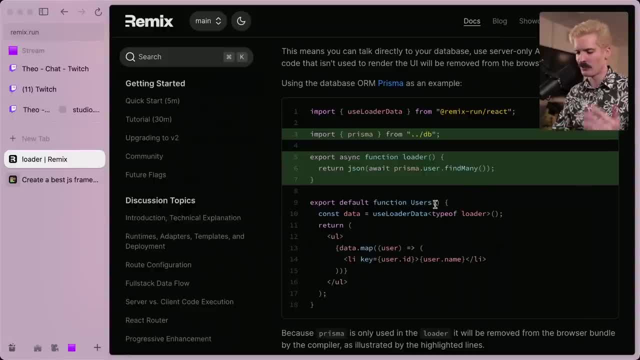 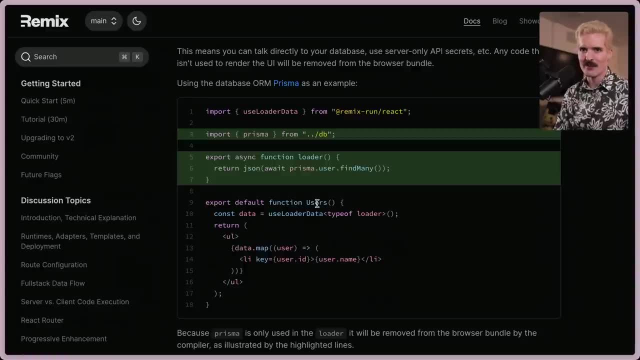 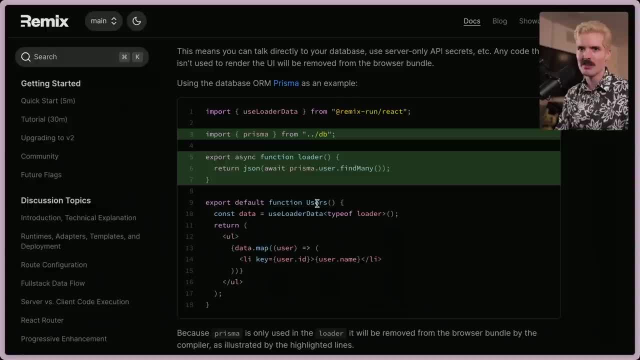 caching the primitives to using web standards more without remix. i don't think nextjs or even react would be where they're at today. i would just never use this framework in a real code base. it still doesn't behave in a way that i consider reliable enough unless you're very, very remix brained your. 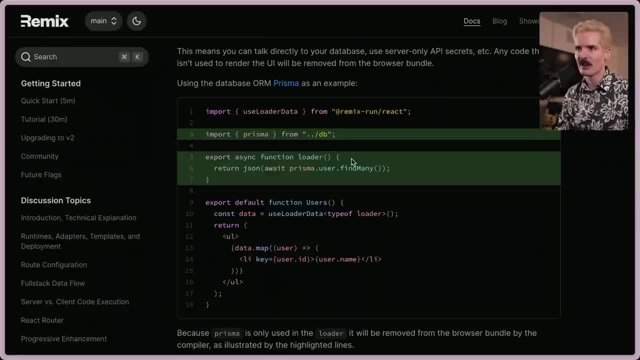 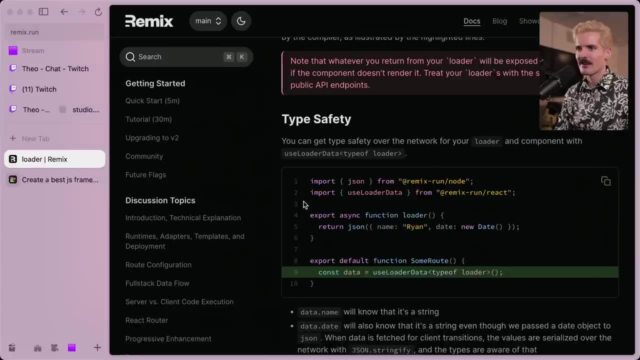 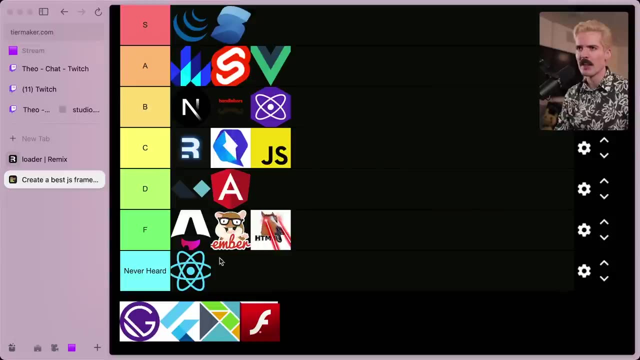 whole team is very, very remix brained and you're not really using actions and loaders as the main layer for interfacing with your application. yeah, those are my thoughts on remix. once again, very important framework for the web, not one i would use. i'll put it on quick tier, i think 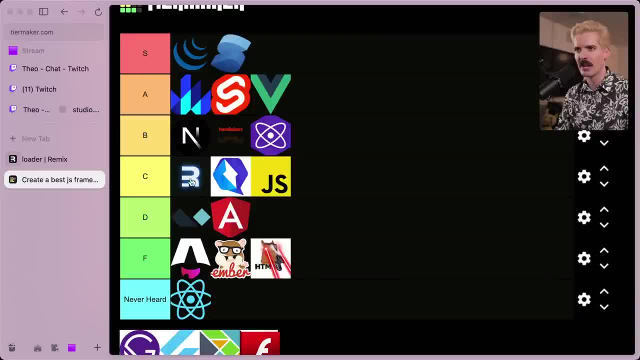 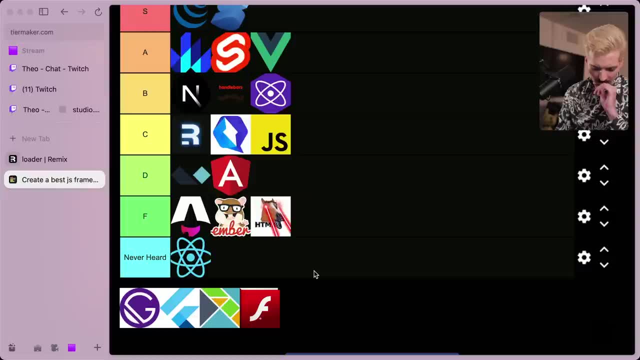 that's fair. also funny how all the things that are behaving like vanilla js- that's goal is to be modern js, but better- and standards- right there, it makes sense. they're all grouped together. oh god, gatsby. oh god, i forgot this was here i. if you're somehow not familiar with gatsby, it pioneered this. 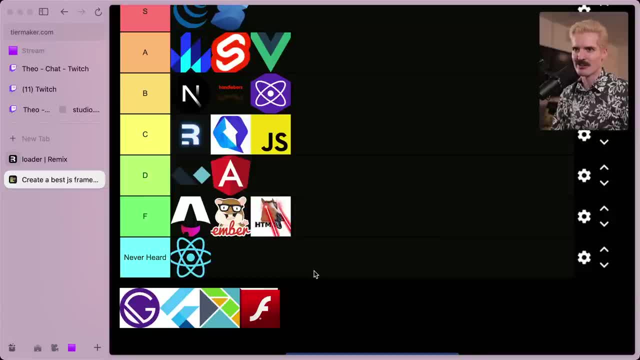 idea of a react framework that generates html pages. so if you wanted a blog in react and you wanted to have html that was cached and would load as soon as you open the page- with seo and all those types of things, gatsby was the first attempt to really do that, and the way they did that was. 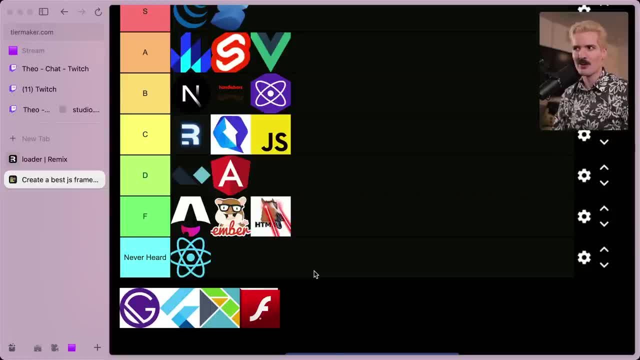 and the way they did that was i, you, not graphql. they built a giant graphql layer to pass data that you would either be through one of their plugins or loaders to get things out of your old wordpress site, or their markdown parser plug-in or any of those other things that would 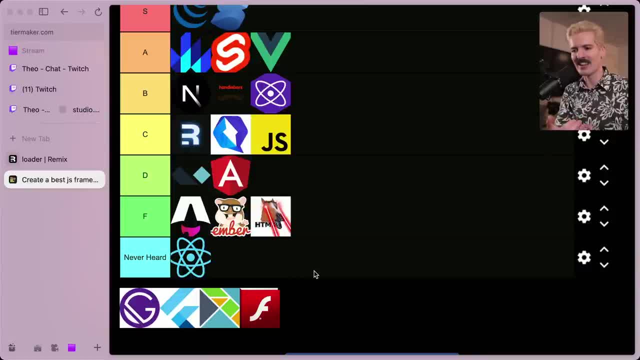 then serve as a graphql schema that you would access in the pages. it would then take all those data that you find in your schema and all the plugins and such. run all of your pages, one at a time. run all of the code for them. figure out what data they're asking for, grab it from that, embed it. 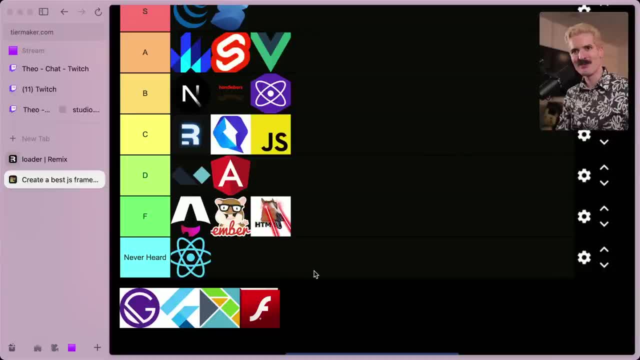 spit out that html as a file and then you'd upload that to a cdn. this is how a lot of these tools work, to be fair, but it was the first to do it and that huge graphql layer in the middle ended up being really painful, like really painful. it was rough, ah yeah, and obviously it has since been. i don't want to say formally killed, but pretty heavily gutted when they got acquired by netlify. framework was dropped in favor of that abstraction for graphqlifying anything, and i think that's where their strengths are. but their strengths as a framework are awful. i mean it is. 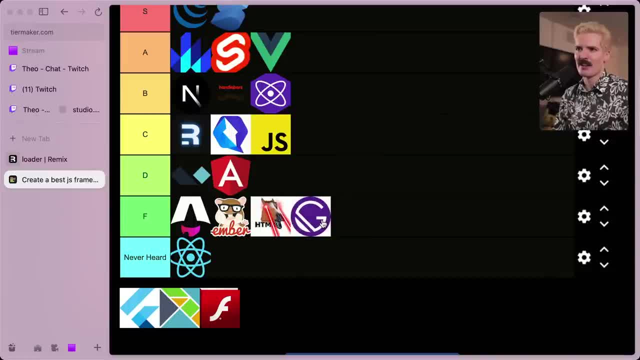 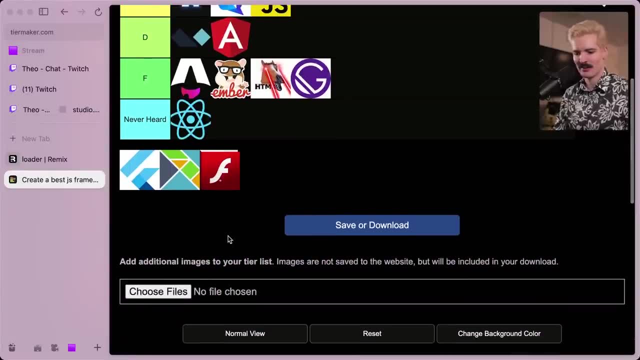 still the javascript. it doesn't have client code still, so yeah, it goes right here. they found the worst possible way to do a react website generator. a lot of people are asking for next. for context, when i made this, i didn't have any of the meta frameworks like next, remix or gatsby, but people 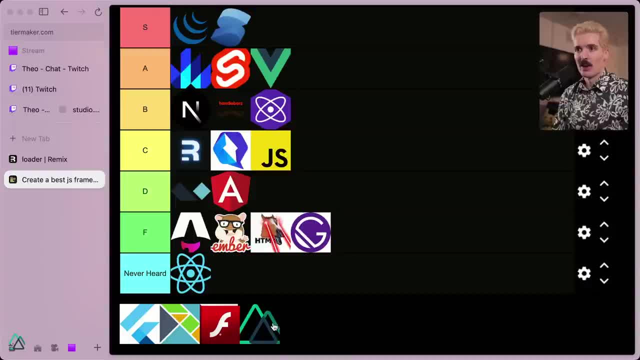 kept wanting them, so i added them in quick. it's only fair to add next as well. no, i'm not adding start. no, i'm not adding svelte kit. i'm not adding all those other things. nuxt exists because a lot of the view community was- i don't know how to say it- other than a bit jealous of what was going on in. 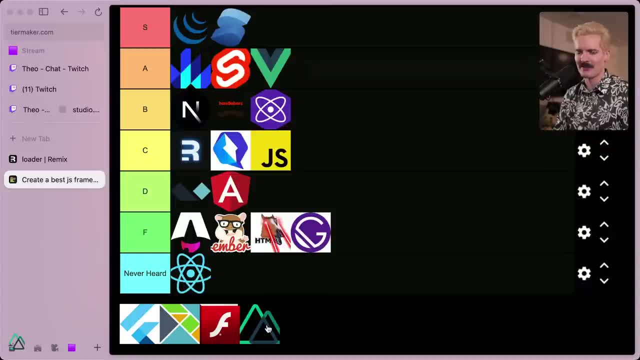 the react world with nextjs and they wanted to enable that level of full stack developer experience within view, and they've done some really cool stuff. in nuxt, they built a plugin system that's full stack, not just back end or front end. we're working on integrating that with 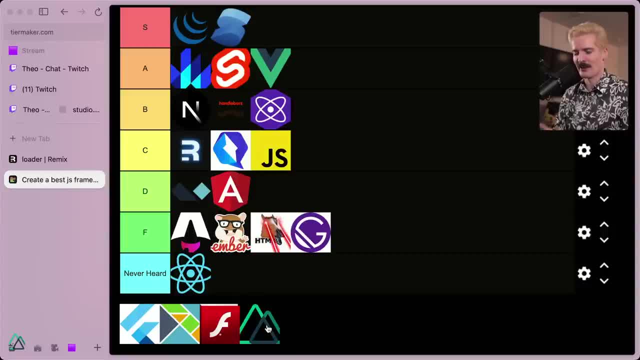 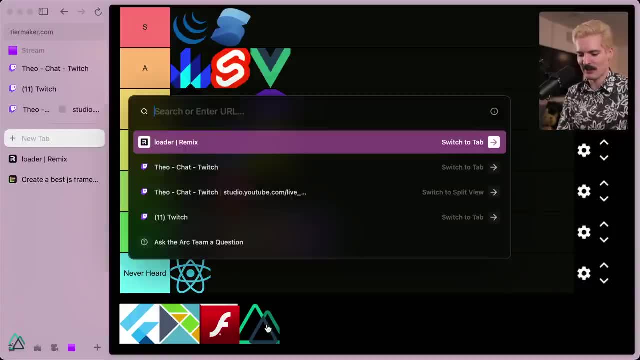 upload thing right now and it's going pretty well. they implemented an actual rpc like solution that uses typescript to let you know when you're fetching data what the type's going to be. i can show that a bit. they have a use fetch helper function as well as the dollar sign fetch for. 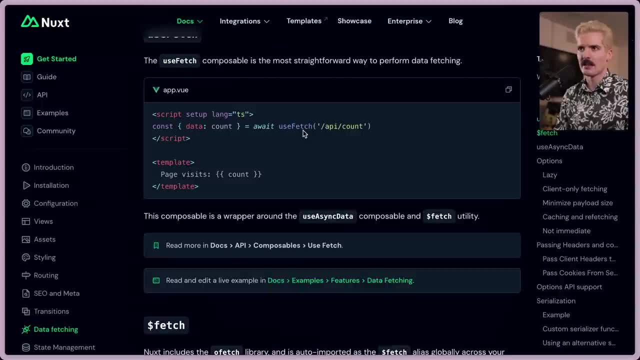 making network requests based on user interaction. and when you call this, it can look at what this endpoint serves, because it's your application and it will grab the type definition from that and give you the correct type for your data. it's still doing some code gen stuff behind the scenes. 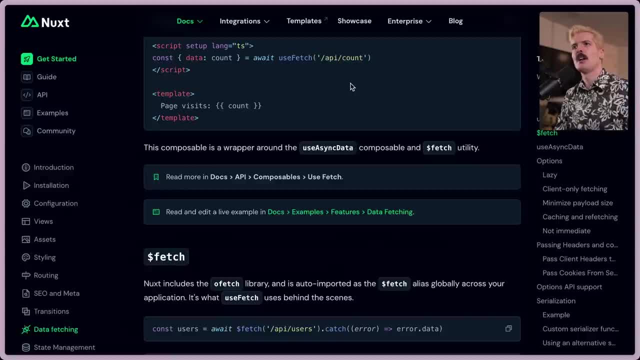 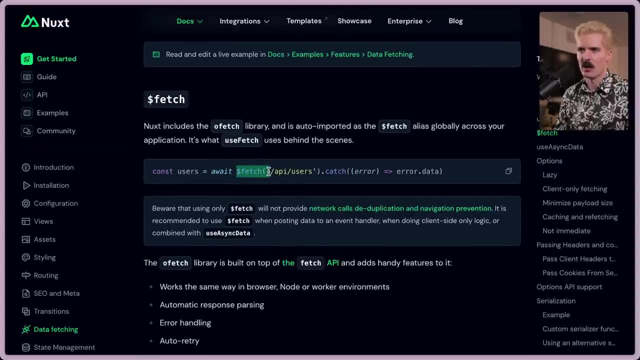 in order to assign the use fetch with this specific input to ace another specific return. but it's pretty nice and as such, they also apply this to their fetch call, so you can use dollar, just their custom fetch. pass it a string and it will now know the type of this response and 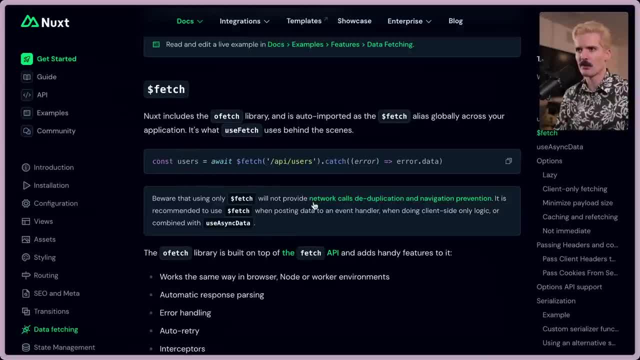 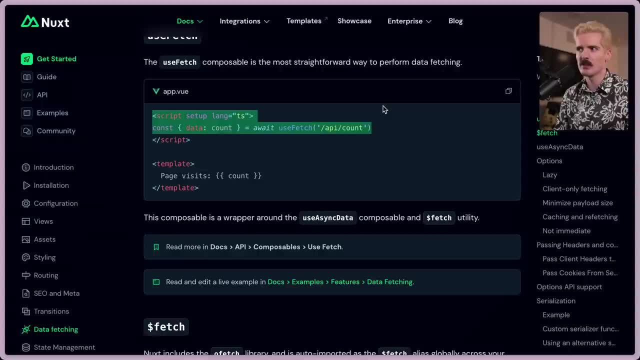 you'll know what users is when you get it. be aware that using only fetch will not provide network call ddupe, which is really nice too. so if you call await, use fetch api count in five places on the same page. it will only call it once, which is one of the reasons that fetch was overridden in the new. 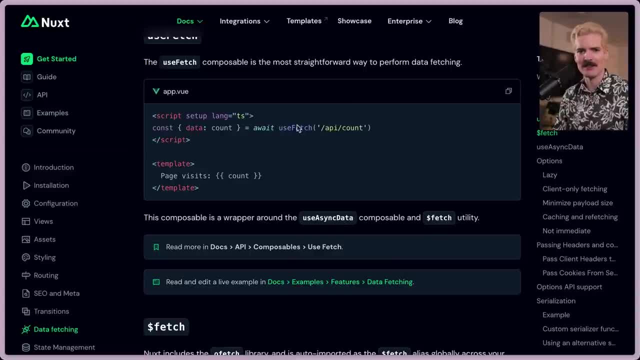 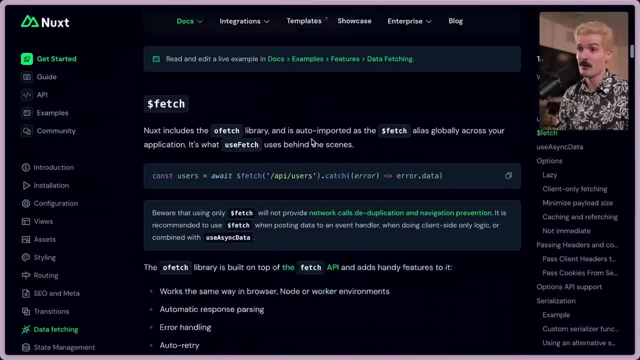 react model. we got everybody huffy, but having it built into the framework in a primitive level it's really nice. i think a lot of these design decisions are great. nuxt is the only way i would personally ever use view and i think it's in an incredible state. every time i see what they're working on, every time i hear an. 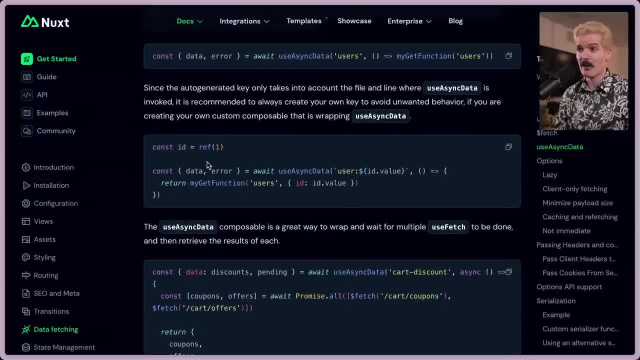 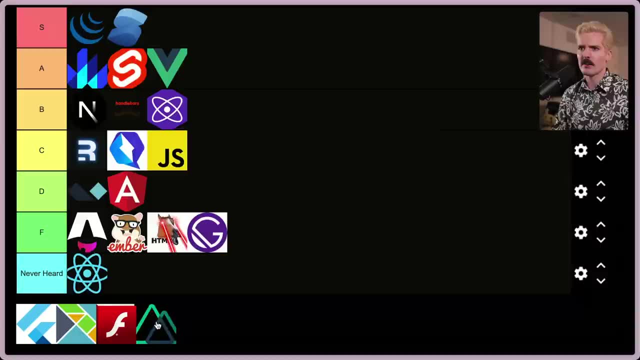 update from daniel rowe or anybody from the next team is getting more and more compelling, to the point where i would argue nuxt is one of the best meta frameworks and i wouldn't think about using view without it as such. i'm gonna put it slightly ahead of you, which also puts it at the highest. 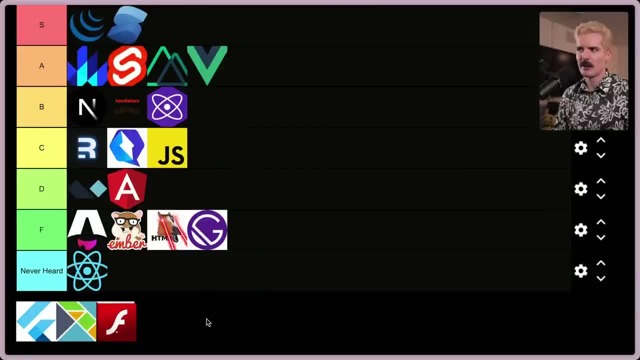 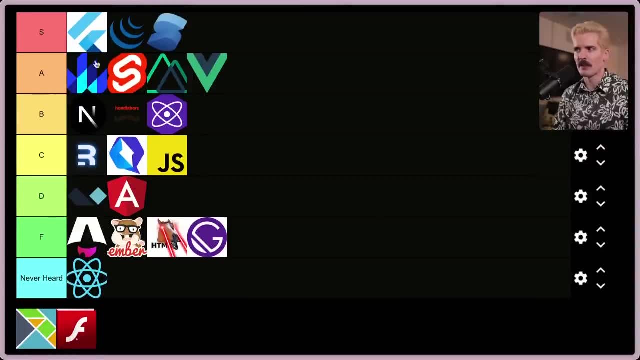 rated meta framework. see why you guys want me to put that there. do i have to talk about flutter now? flutter for web instant s tier. it's the only thing that fully escapes from the web primitives and you get further away from web standards. things get better. who needs the dom? who needs a button? 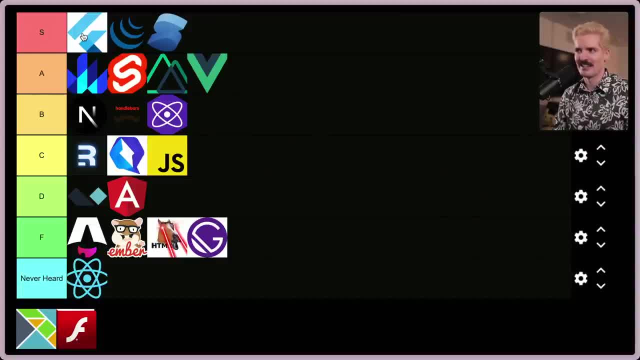 element when you could just render everything in the canvas. it's great. web standards, web schmanders- come on. nobody needs those screen readers. those are so 2012.. come on, yeah, don't use slaughter for web. even my die hard friends will not recommend for web, like the people i know who are the hardest. 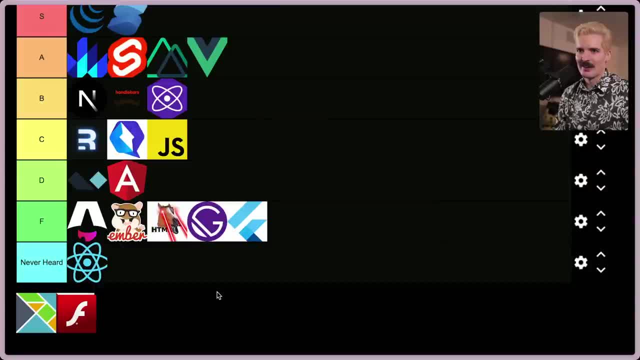 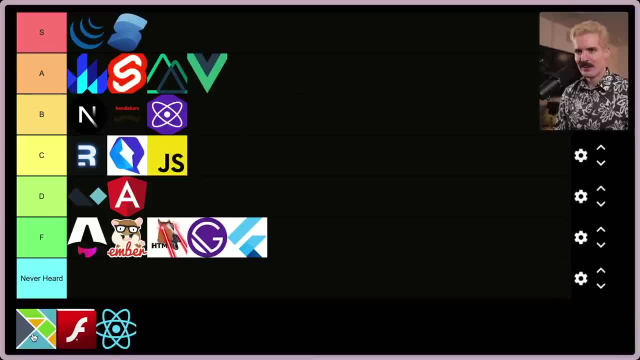 core about. they will tell you not to use it. and now we have our last two. i should give react a real score at the end. i'll do that. so let's do these two and then i'll actually talk about them. and talk about react. elm's an interesting one if you're not already familiar with this chaotic. 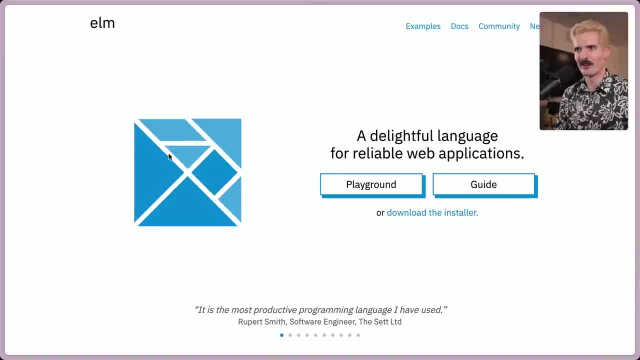 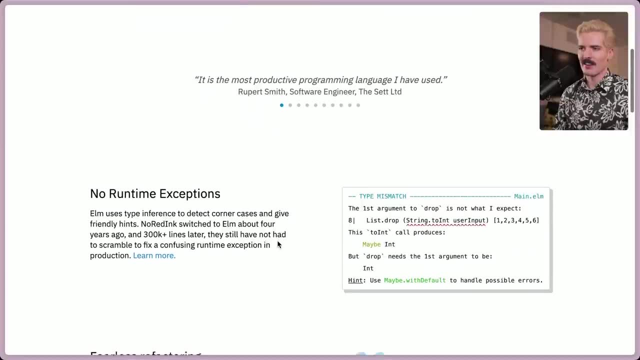 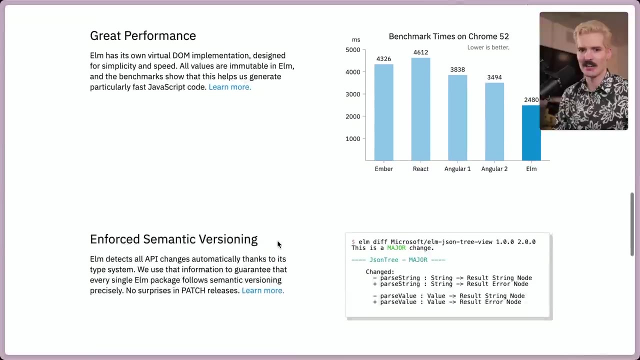 logo. i wouldn't be surprised, because i didn't know that was elm's logo until i went to go find it for this. apparently it's blue. now that's a nice little interaction. elm's interesting because, more than any of these other frameworks, elm is a language and they're very aware of that. they're not pretending not to be. 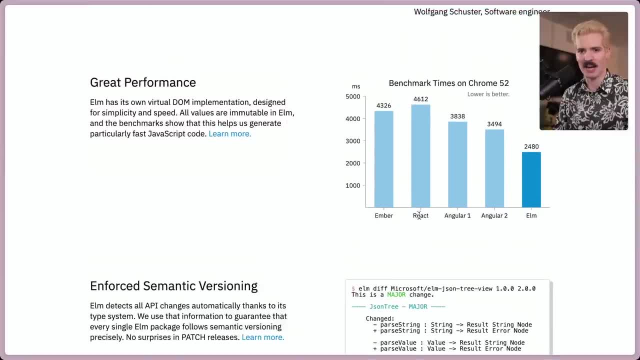 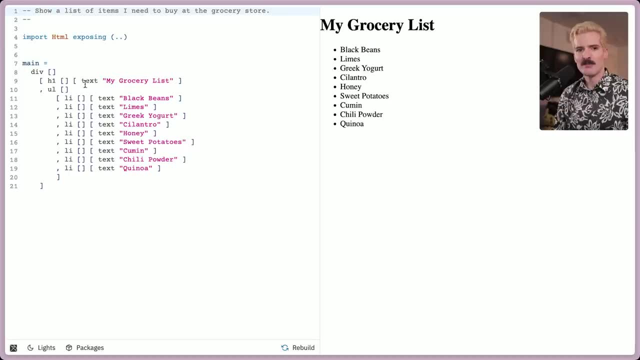 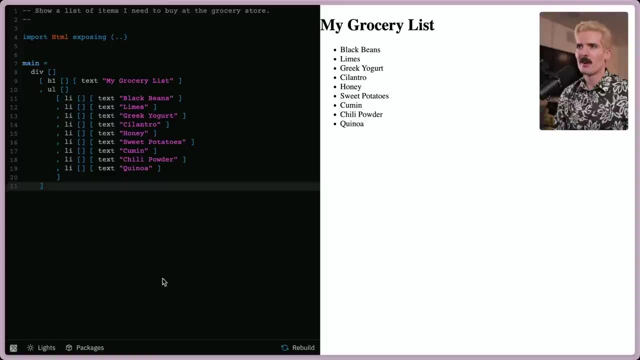 the thing is telling that their benchmarks are against ember react, angular one and angular two. i elms not gotten much love for like five plus years now. so here is an example. markup syntax is weird. it's very nested and vertical, just a dark mode. wonderful, i guess it's dark mode for this half. 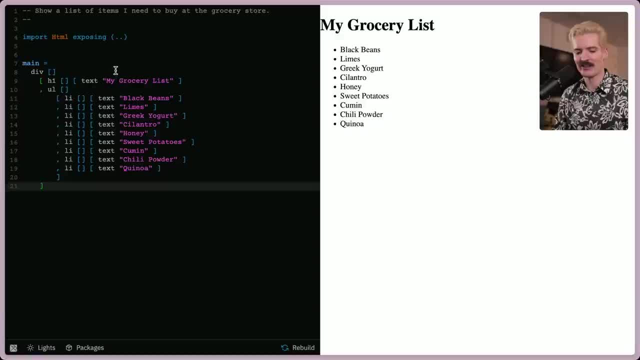 so yeah, it's weird. i don't love it. it's actually very similar to swift ui if you've used that, but it's very strange and having to manually assign text. first you pass it an empty array which says this doesn't have children and then you pass it another array which says this is the text element. 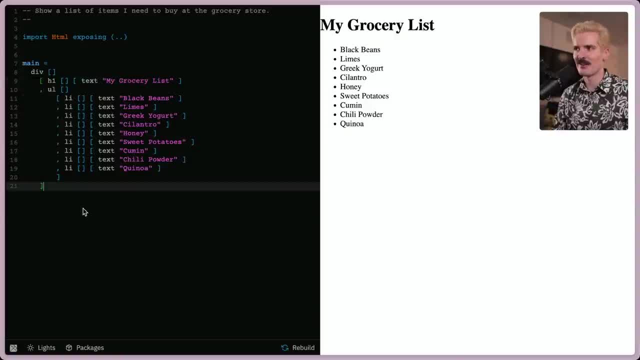 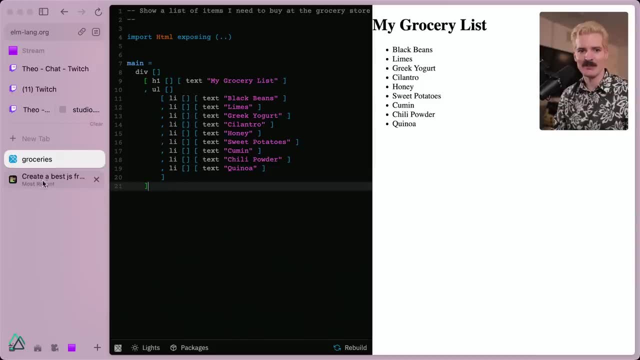 and comma means this is the next element. it's weird. i don't love this syntax, like as the fp guy. this is too far for me and as a result it has not seen much adoption. it's hard to give elma rating. it's kind of like rating haskell, where it's just like it's cute. i get why people like it, but nobody. 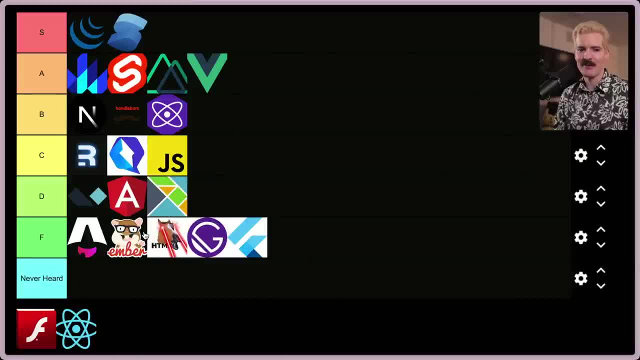 actually uses it. i'm gonna deter it. and now for flash. flash is incredibly based no ios support. anyone can use. it. works on android. crazy touchscreen friendly. all of the best games ever made were made in flash. we're talking impossible game. we're talking somebody in chat, excuse me. flash on android. 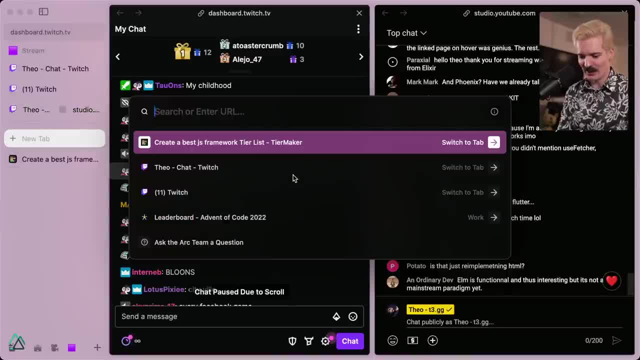 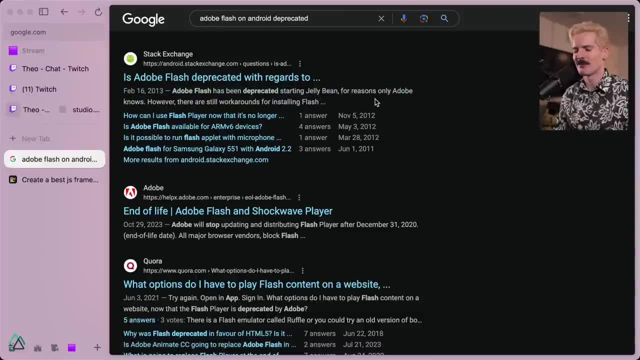 existed. you, sir. your zoomer is showing this was on, i believe, froyo. it was literally. two years later on, jellybean adobe flash stopped being supported on android. it lasted for two android releases because it was such a bad experience and nobody was using it. it literally only. 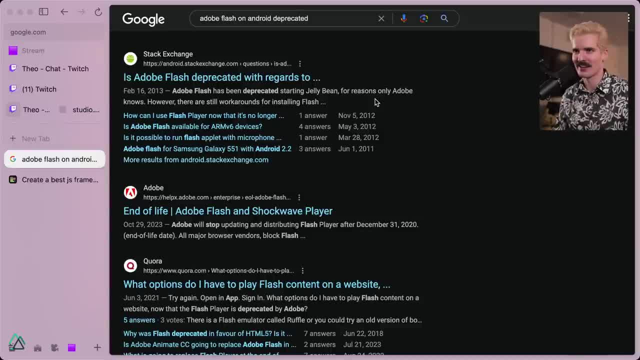 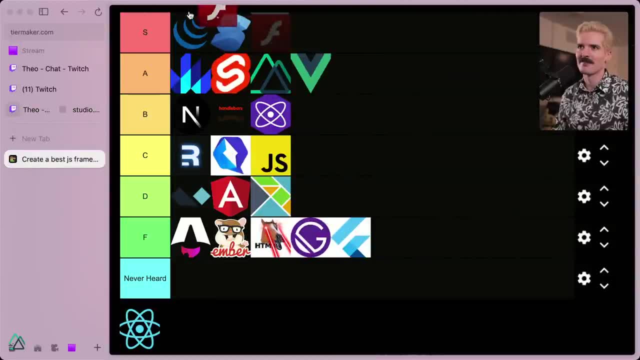 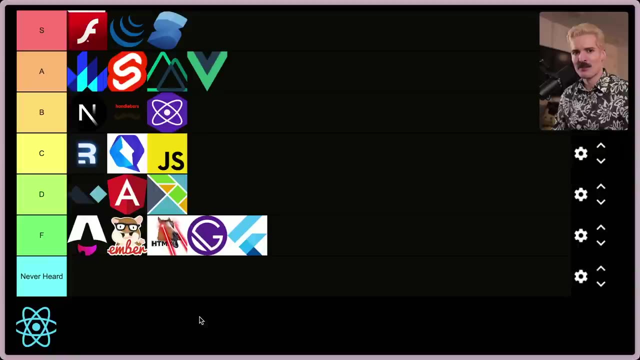 happened, so that they had points against the apple users. that was it. it was awful. and all of these ry, flash goes in the base tier. yeah, we'll put flash as number one. that's only fair. and now for the framework that brought us all here. io react a lot. so much of my success, both as a 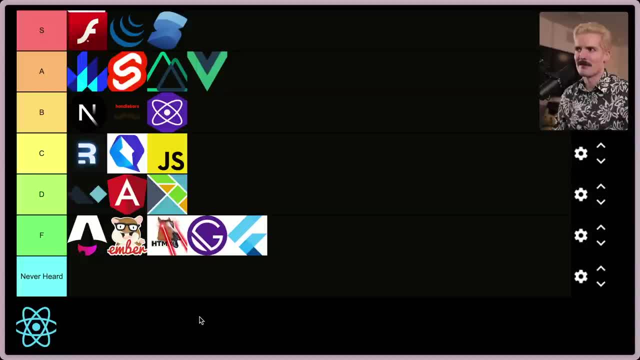 developer and as a creator, has come from this framework. so i am absurdly biased, like absurdly biased, here. react is the only framework here that has continued to meaningfully evolve over a window as long as it has been around, for angular is getting there now with the most recent release, but angular is historically unwilling to change.